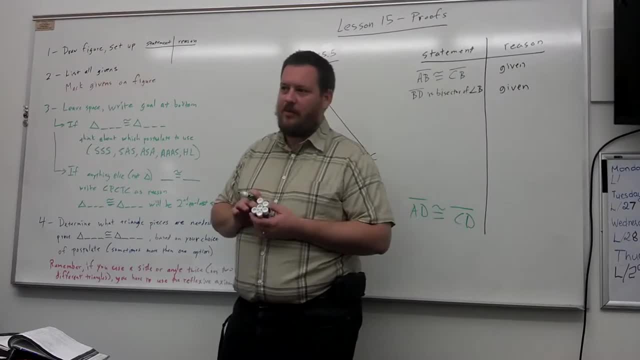 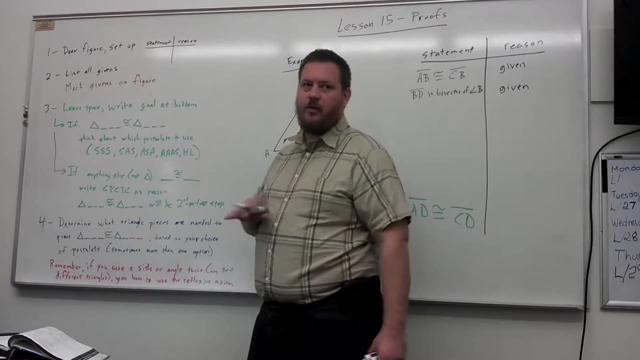 Now, if you took a course that was specifically all about geometry, there would probably be more to it than this. This is the extension that we're going to do. All the proofs that you will have in this class should be solvable following these steps. 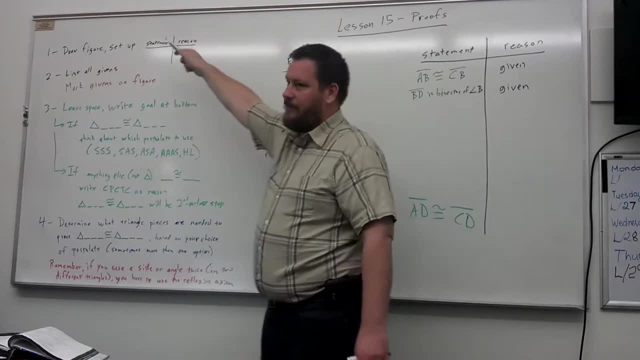 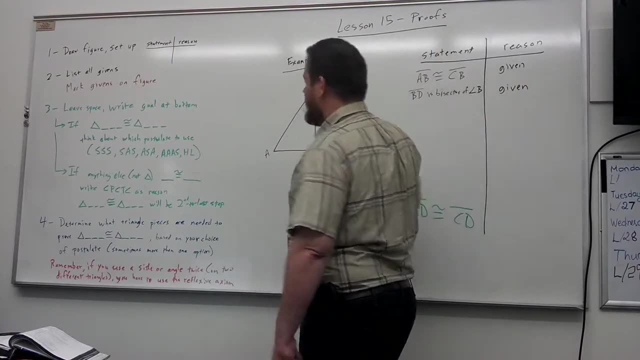 First of all, draw your figure and set up your statement and reason. two-column format. These are called two-column proofs, by the way, And this is why: because we're going to make two columns. So the first thing you want to do is draw your figure and set up your two-column T. 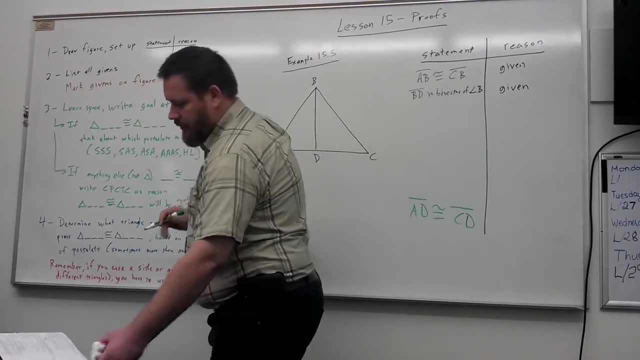 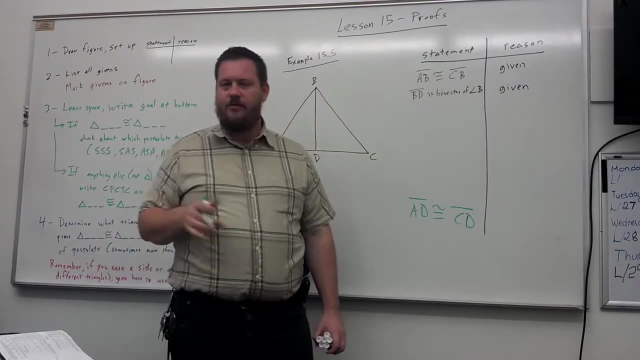 Then you have this: Then list all your givens And the problem will tell you that. So it'll say: given blah, blah, blah and this, and sometimes, usually there's two, maybe three givens, Sometimes one, sometimes more than three, but usually two or three givens. 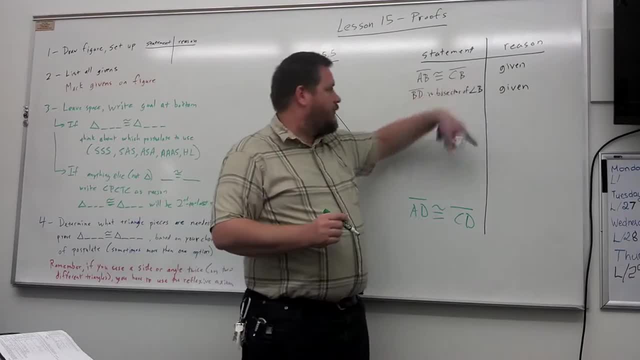 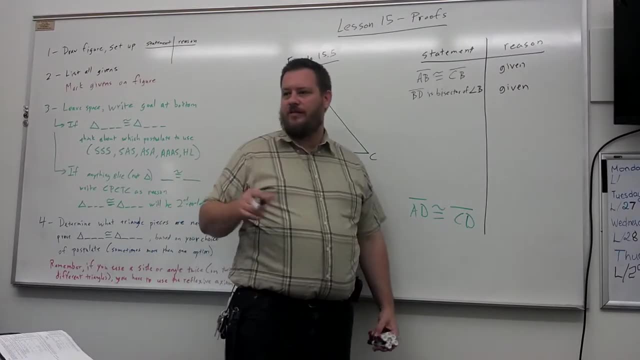 And so you can start right off the bat by, just when you set up your T here with statement and reason, just make the first couple lines given, because that's information that the problem has given you. So in example 15.5, I 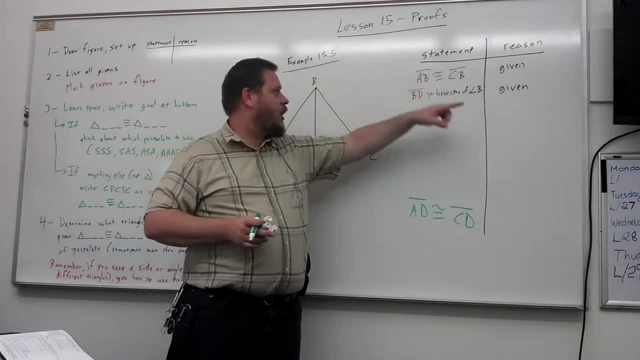 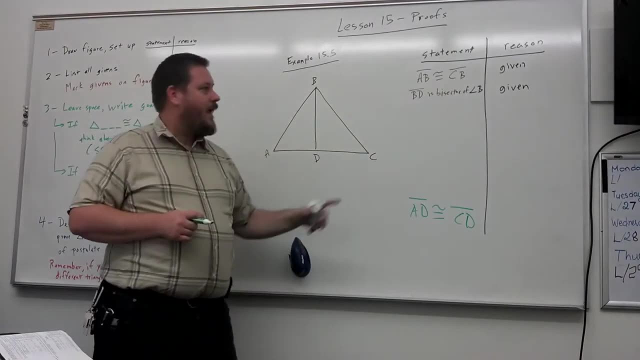 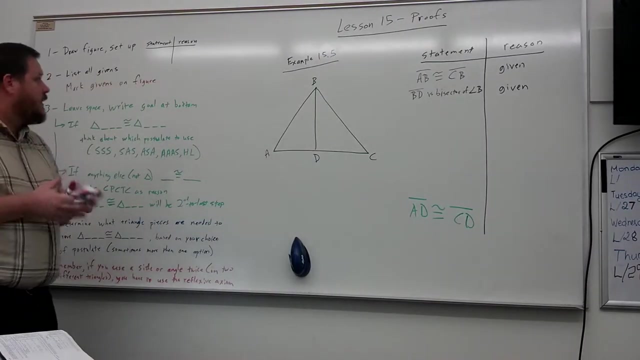 I copied the picture from the book. I set up my two columns and the book tells me that line A B is congruent to line C B. It also says that line B D is the bisector of angle B. So what I can do is I'm going to label that on my figure. 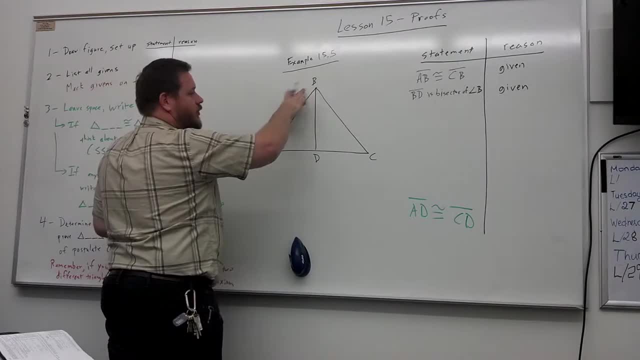 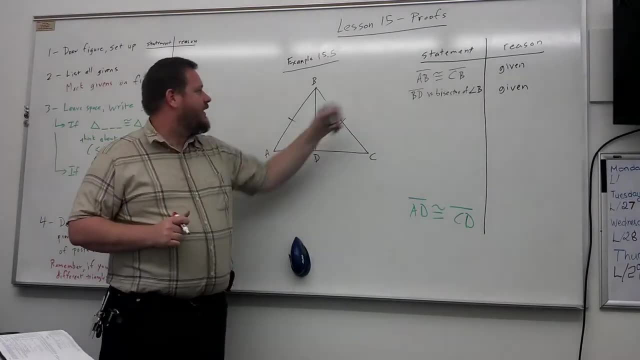 So A B is, this line segment is congruent to C B, So I'm going to put tick marks right there, Because that's it. That's the information that I was given. Now, the other thing that I was given is that line B D, that this line is the bisector of angle B. 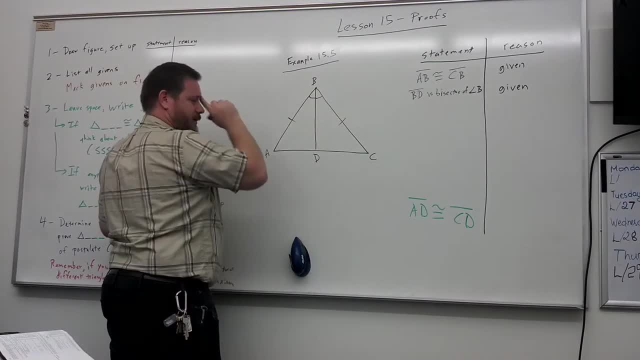 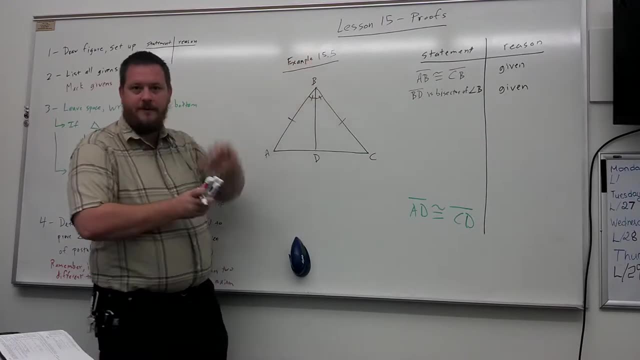 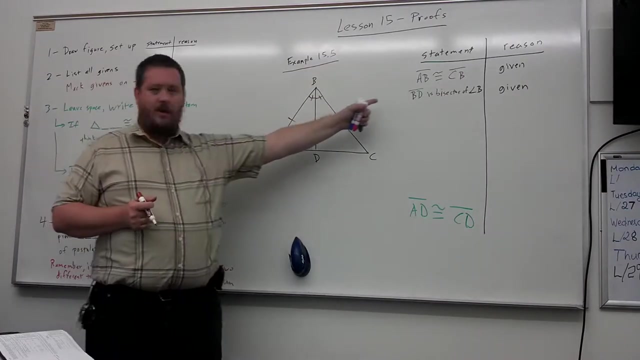 What that means. that means that that this line cuts, cuts this angle in half There. so now I can, already now. so I've already made a conclusion based on what I was told. So what I'm going to, what I'm going to say here, is I'm going to say that 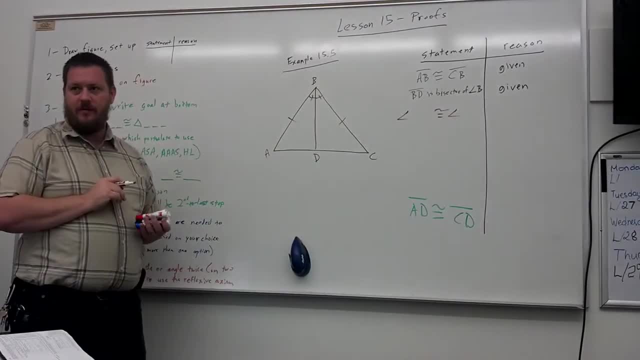 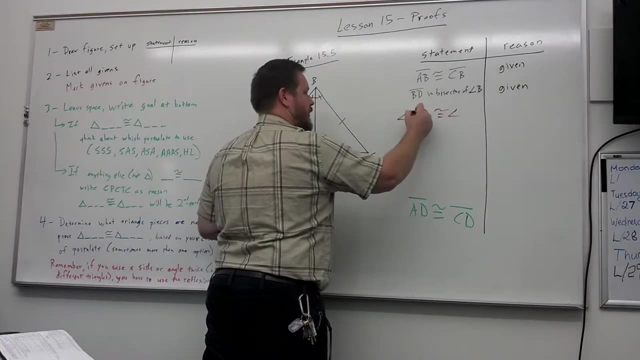 which two angles are congruent. therefore, A, B, C, D, I get A B, D And since I went in this order outside top down the middle, I need to do the same order for the other one. 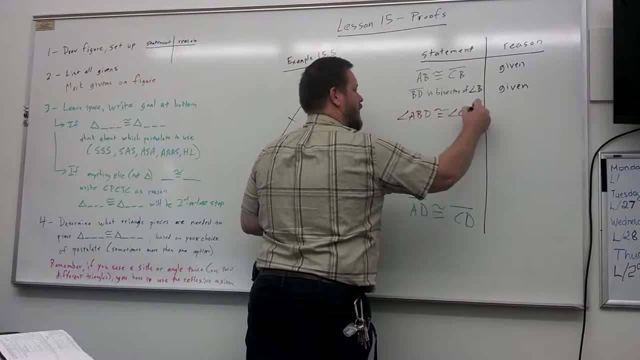 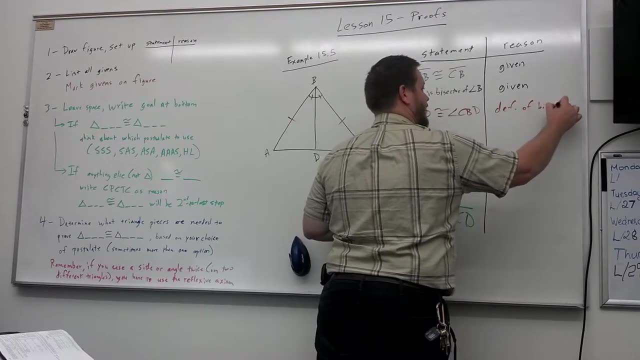 C, B, D, And that's just because that's what the definition of a bisector is: Definition of bisector. And for the, for the reason, for the reason, for the reason There's a, there are a couple things that are that are just standard things to do. 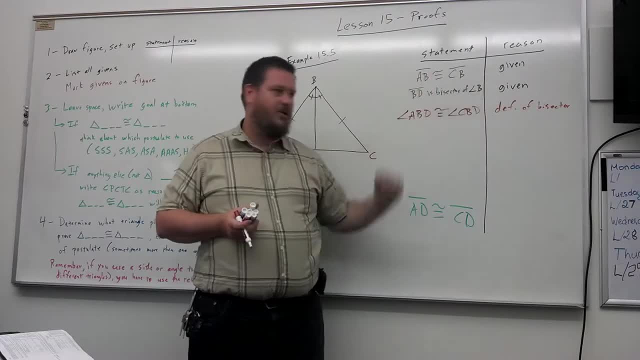 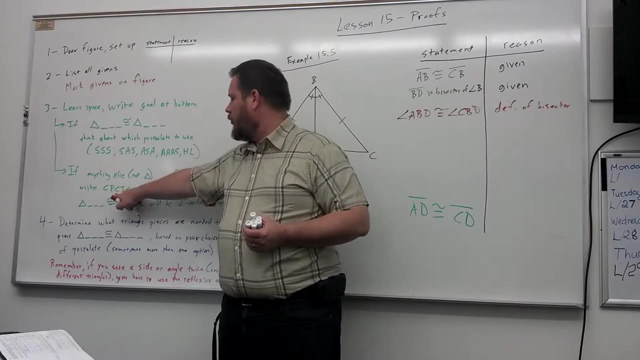 Like. the word given means that this was given to you in the problem. The acronym C, P, C, T, C, Congruent or corresponding parts of congruent triangles are congruent. Those are things that are used all the time. 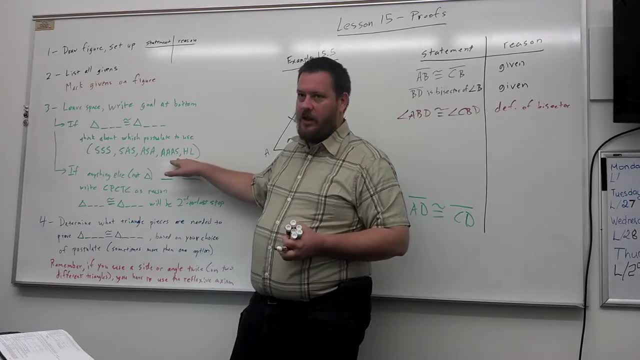 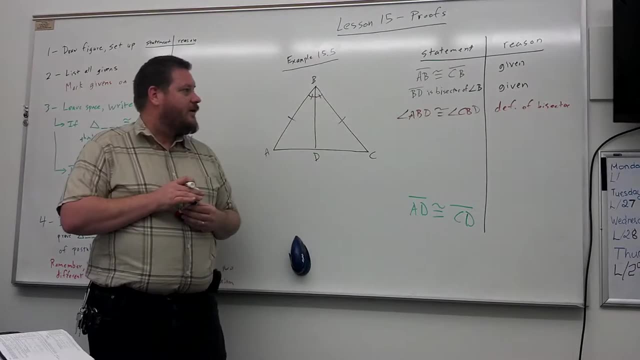 It's the same with the postulates. the triangle congruency postulates The reasons why a triangle can two triangles can be congruent. So those are some of the standard ones. The otherwise just Don't get hung up on exactly which words to use. 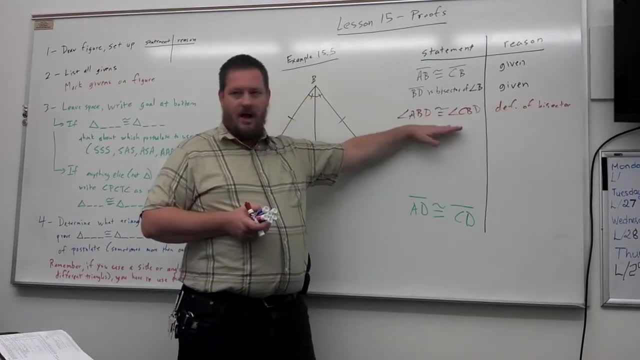 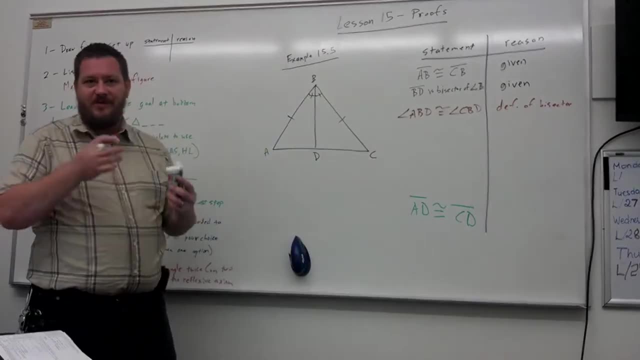 Put something here that tells me that you know why this is true Sometimes. so like definition of a bisector, definition of a midpoint, definition of perpendicular, You know just some, some things like that, Or maybe, maybe things are corresponding angles. 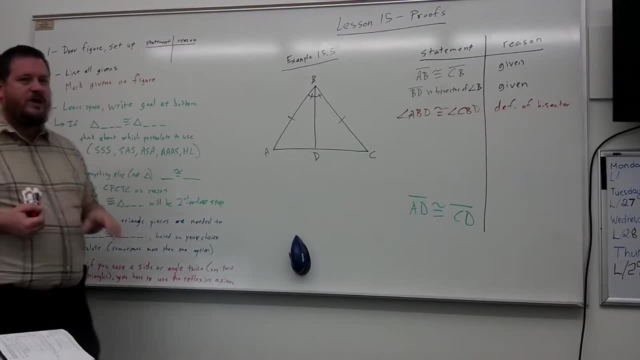 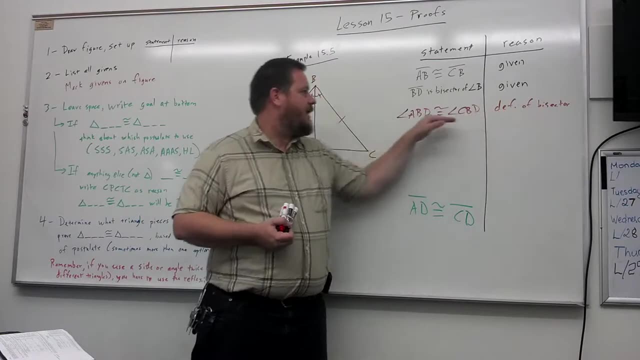 Et cetera, et cetera. So don't get too hung up on using the right words here. Just make sure you have a reason, Make sure you know why you can say this. So that's all the information that I've been given. 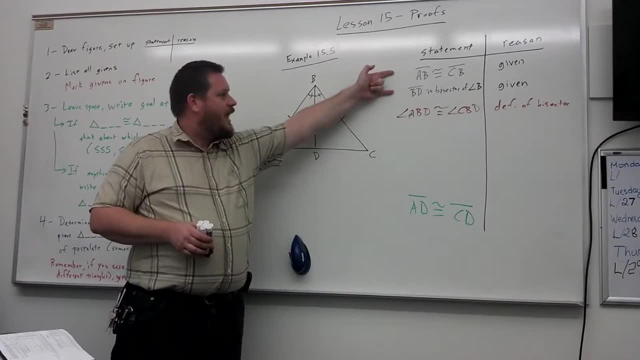 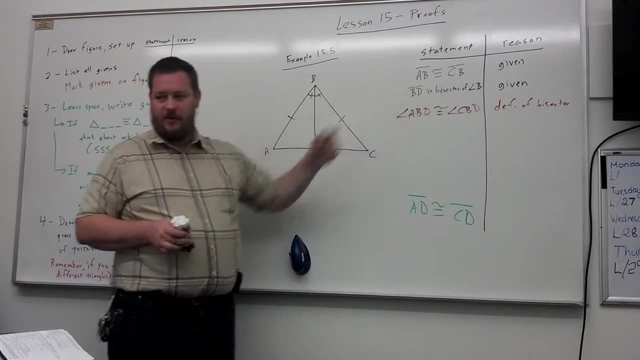 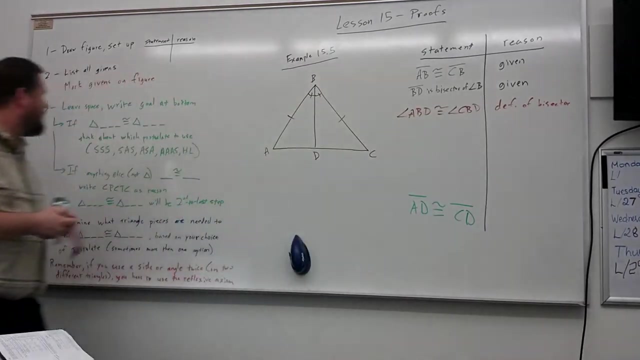 I wrote down what I was explicitly told, And then I also wrote down what I a conclusion that I drew based on this statement that I was given. So the next thing I want to do here is I want to leave some space right here for my additional steps. 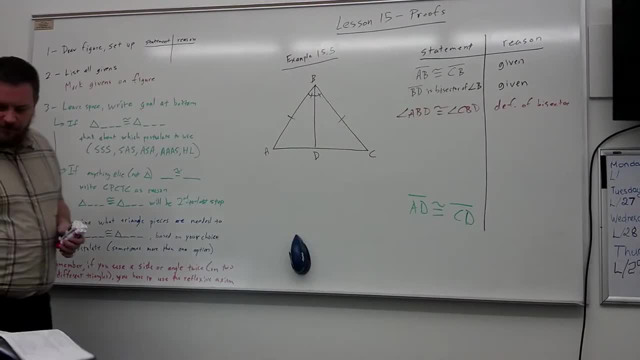 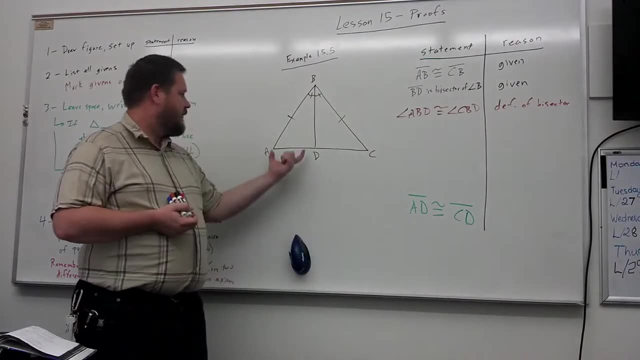 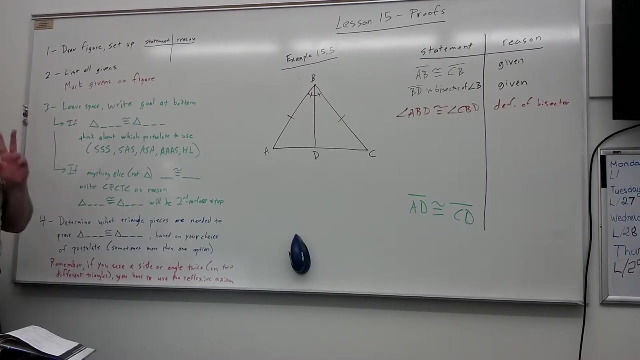 And I'm going to write my goal at the bottom. Now this particular problem. it is asking us to prove that line AD is congruent to line CD. This one is congruent to this one. Now, the types of proofs that we will be doing in this class will fall into one of two categories. 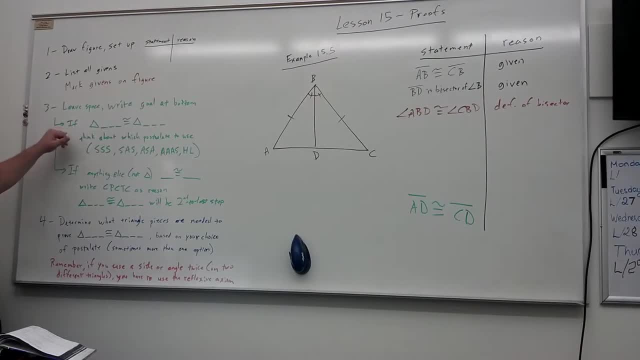 In one category of proofs is that we're trying to prove that this some triangle is congruent to another triangle, And this is not one of those, So I will talk about this one on the next example. This one is: this is the proof where we're asked to prove something: that two things that are not triangles are congruent. 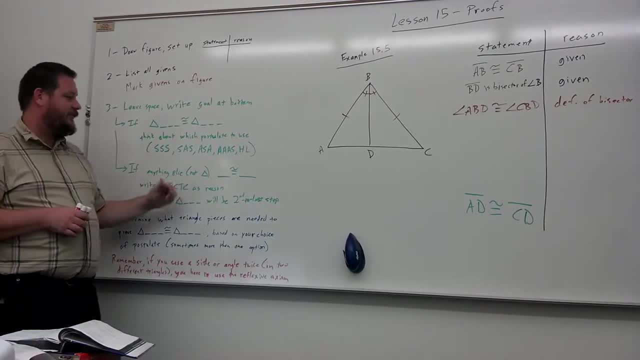 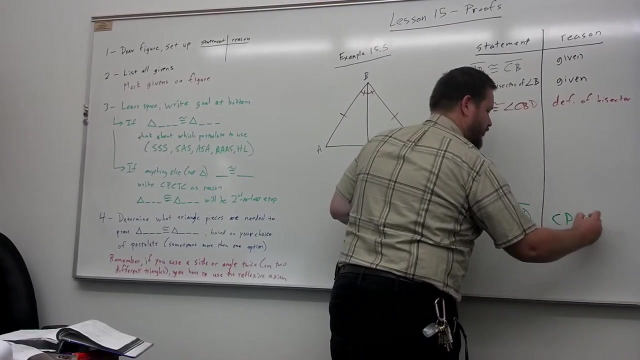 So anytime you have you're asked to prove that anything else something is congruent to something that's anything else but a triangle. here's how those will end up. That means that whatever you're trying to prove, the reason for it is going to be that they are corresponding parts of congruent triangles. 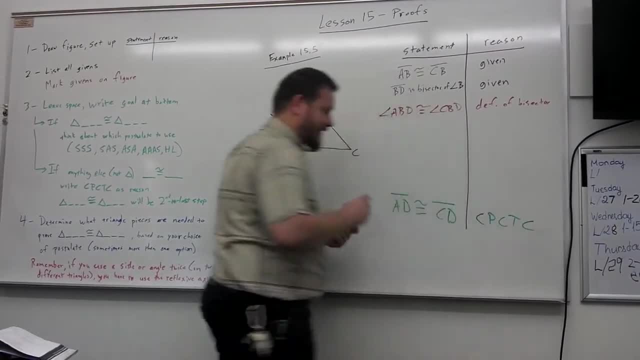 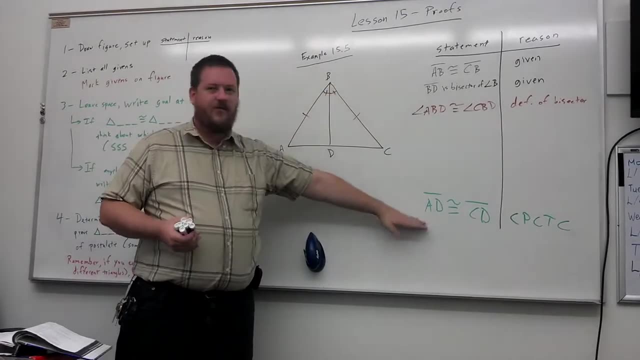 And corresponding parts of congruent triangles are congruent. That's going to be the reason for this, And the idea here is we're given information at the beginning, we're asked for something at the end. so we're kind of trying to say, okay, based on this, I got this and based on the fact that I'm proving this. 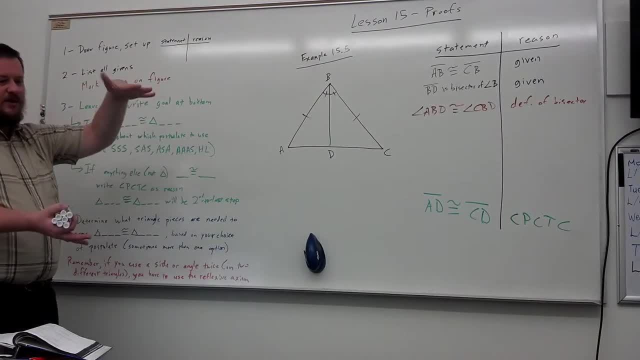 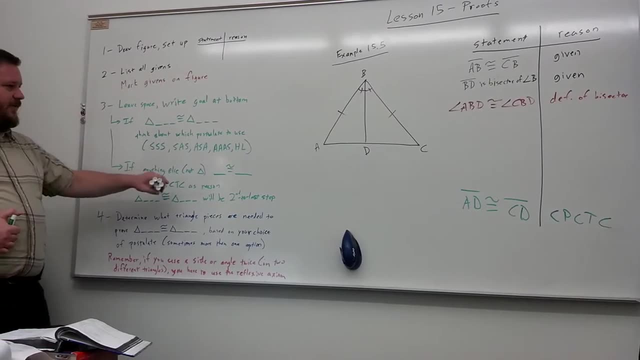 I know what my next to last step is, and it's going to be to figure out the middle part: How to get, how to get from there to there. Okay, so we're trying to prove that something other than two triangles are congruent. 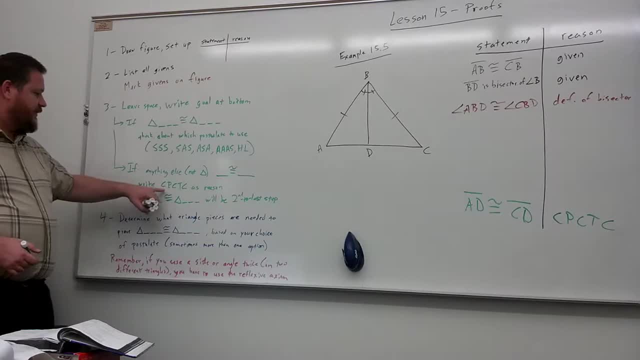 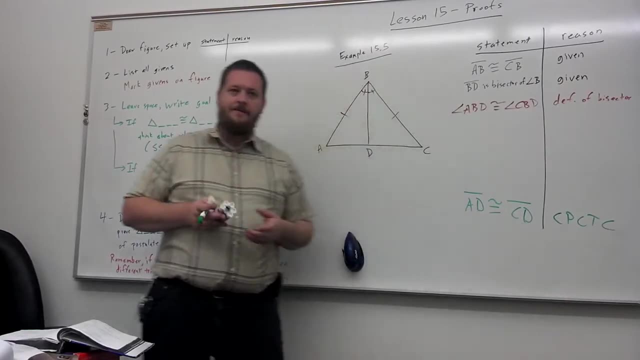 So I go ahead and write that at the bottom, And I know that CPCPC is going to be my reason for it. And if, if these two things line AD and line CD, they are going to be corresponding parts of congruent triangles. 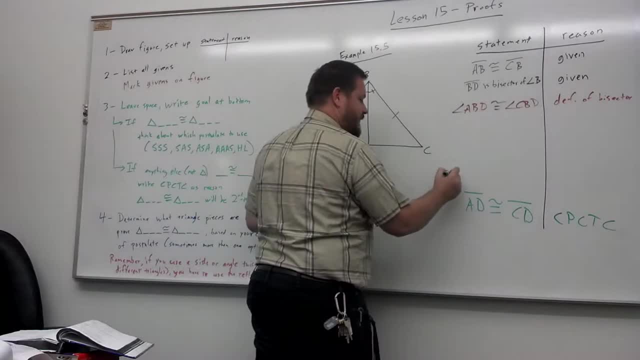 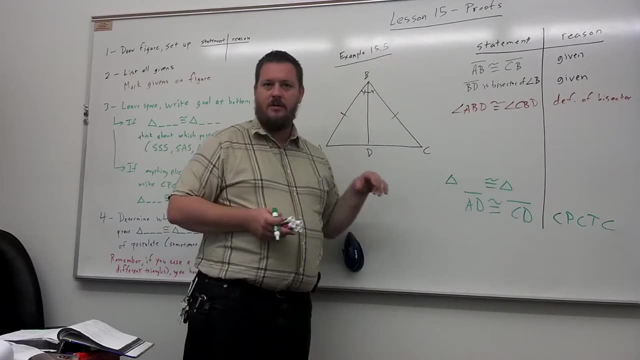 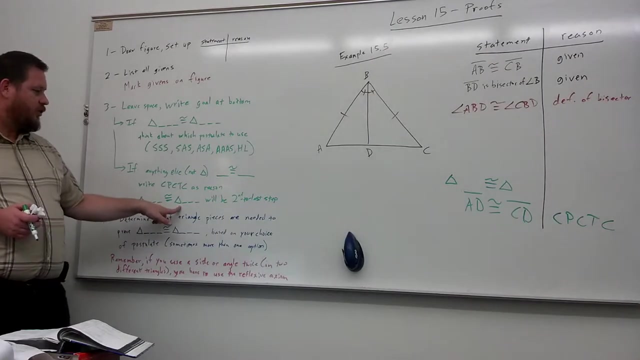 therefore my next previous step. I need to be able to say that two certain triangles are congruent. I don't know what they are quite yet, Me Okay. So proving that two, two triangles are congruent is going to be. 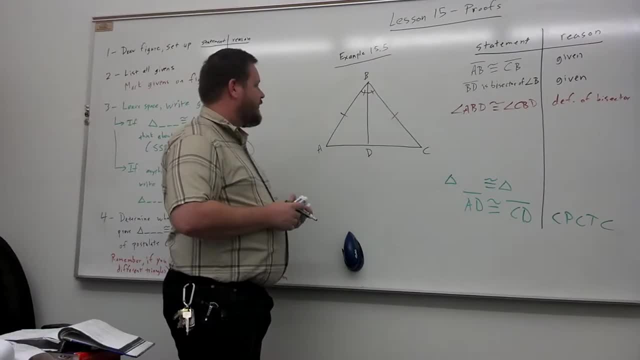 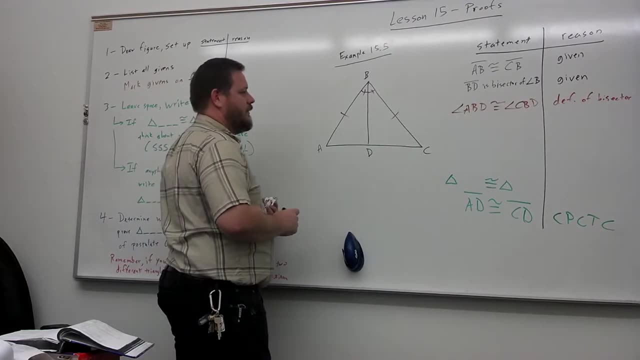 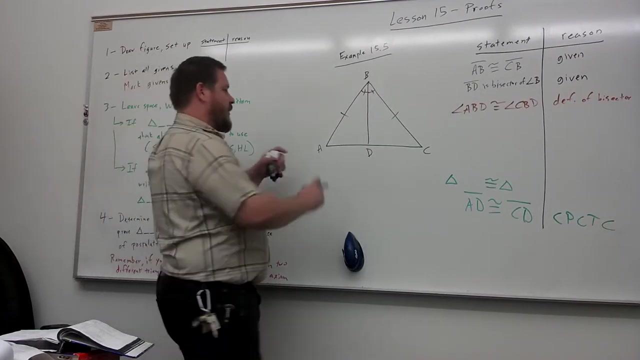 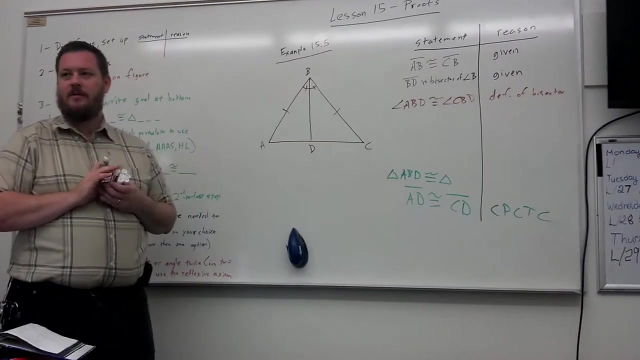 is going to be your second to last step. Now, looking at this, which two triangles do you think they're going to be? Jack ABD And DBA C DC. Um, right idea, wrong order. If you talk about triangle ABD, what is the other triangle? 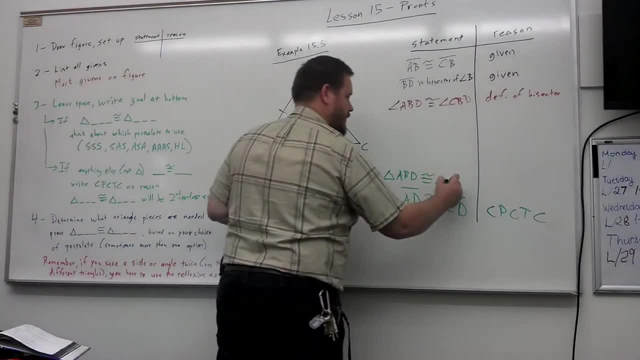 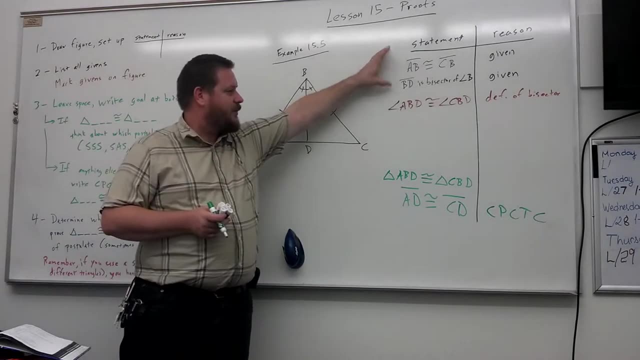 CBD, CBD. yes, All right. So now we've- we've set up our skeleton, We've set up the information we were given and what the obvious thing was from that, And we've set up where we need to end up. 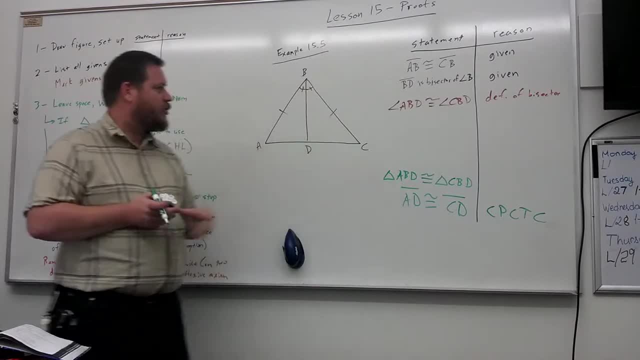 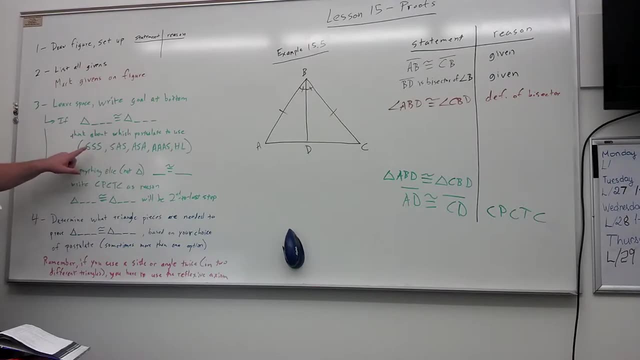 And the way to get here is by proving that these two triangles are congruent. So now what we have to do is figure out which postulate we're going to be using. Are we going to use it? are we going to say that these two triangles are congruent because of SSS, SAS, ASA, AAS or HL? 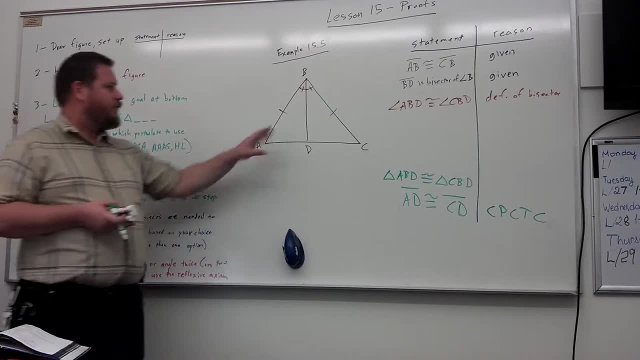 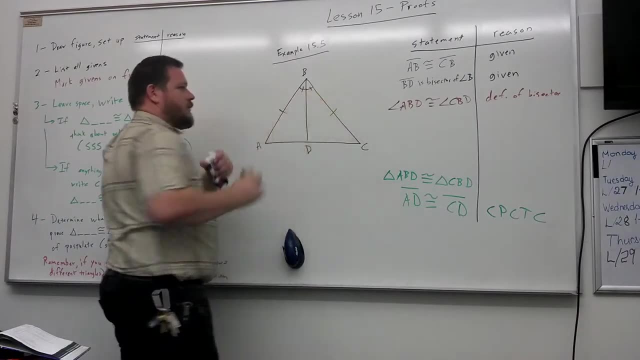 And so we need to figure out which one of those things is going to work To prove, to prove these two triangles. Now what we have is we have a side and we have an angle. So, right there, we're probably not going to be doing this one. 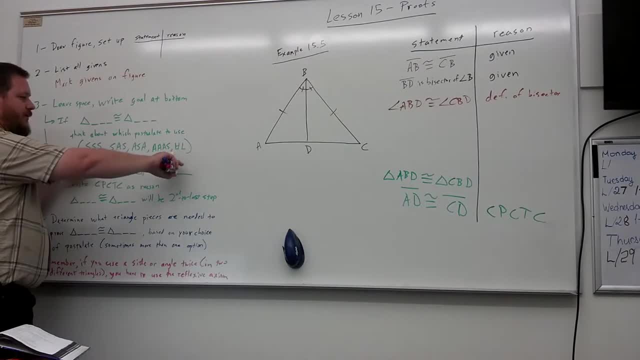 We don't know that, the right that they are right triangles. We're probably not going to use HL. It's going to be one of these And usually, usually, you only have to use this one if one of these two doesn't work. 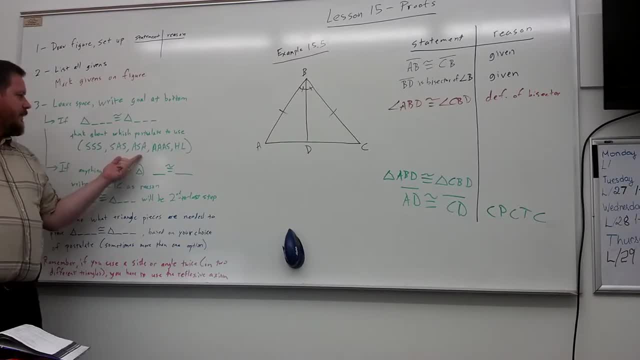 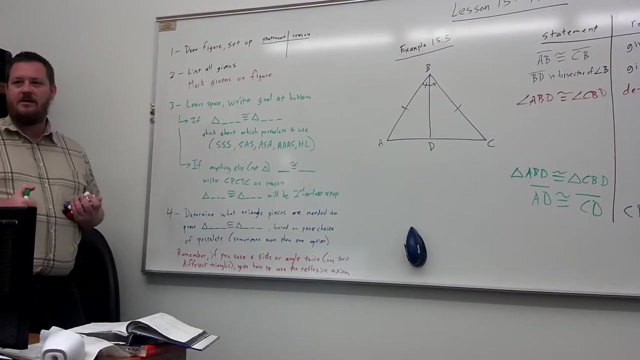 So let's, are we likely to find the side, angle side or angle side, angle, Side, angle side, Side, angle side? Which brings us to, by the way, what I have pinned down here, if you can see it, But if you're going to use a side twice, a side or an angle twice, like once in each of two triangles, 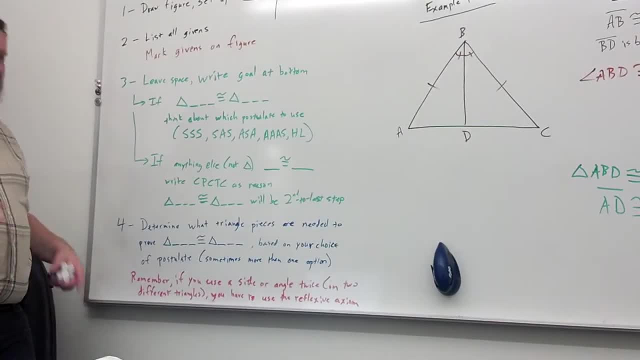 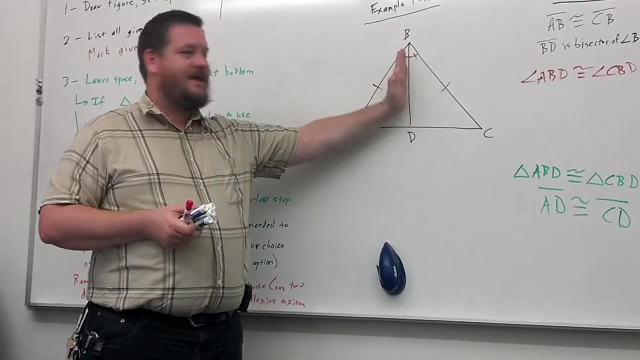 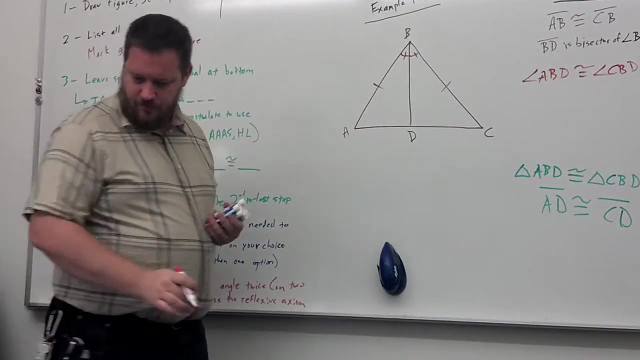 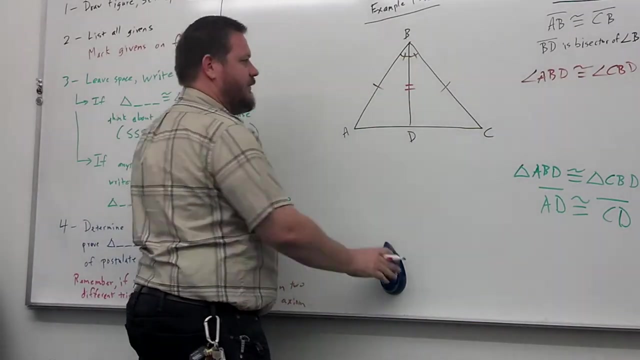 you have to specify that it is congruent to itself And that's called the reflexive axiom Because we're going to use, because line BD is in both triangles. So what you do is, if I remember correctly- I think I could just do two marks like that- 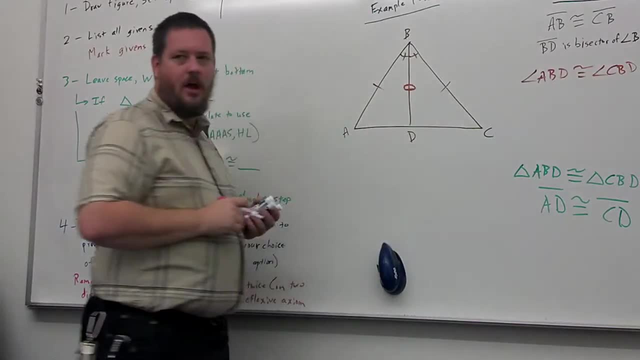 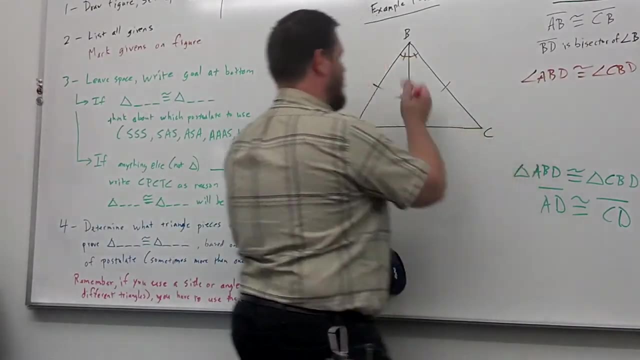 Sometimes the other way to do it is just put a circle on it like that. Either way, the picture is for your benefit. So this one here. I'm going to use line BD twice: Once in this triangle, once in this triangle. 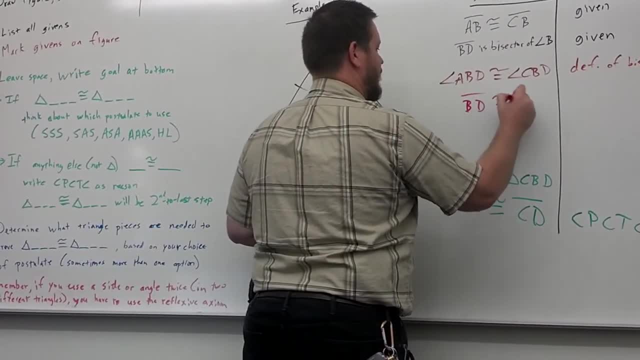 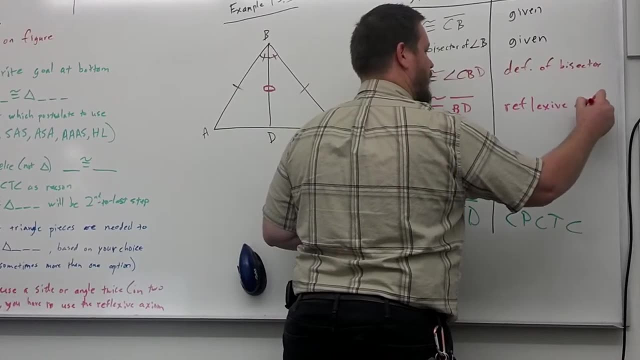 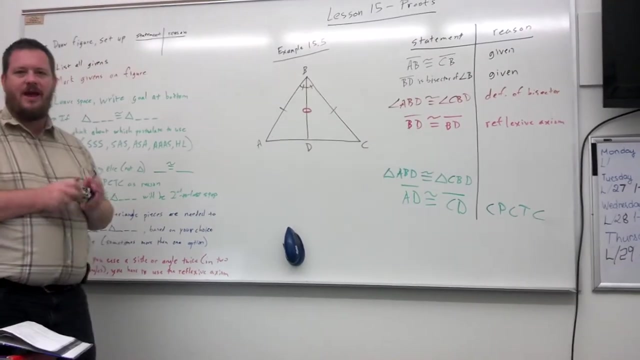 So I need to say that line BD is congruent to line BD And that's called the reflexive axiom. You won't be using that in every problem, but it's often. it happens often enough that you want to make a note of it. 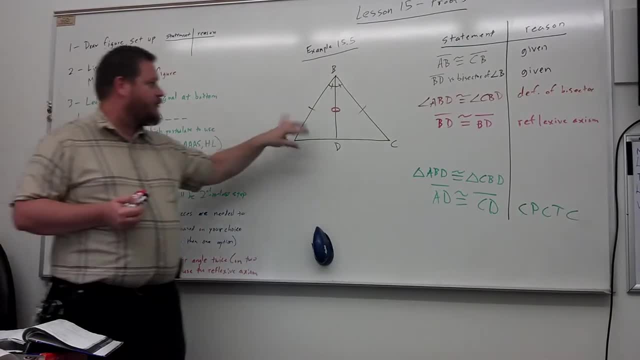 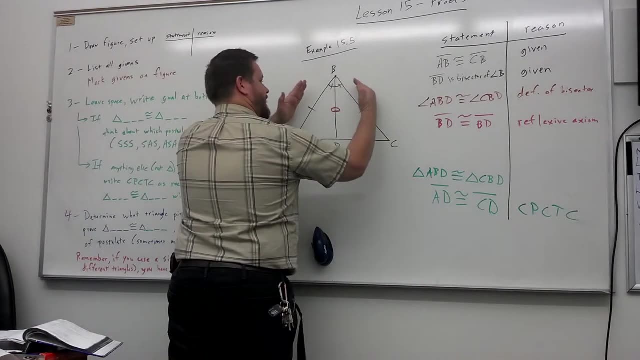 Okay, so do now. do we have enough to say that the two triangles are congruent? For one of these reasons, Yeah, Yes, We have this side and this angle and this side. Now we have to make if we have two sides and an angle. 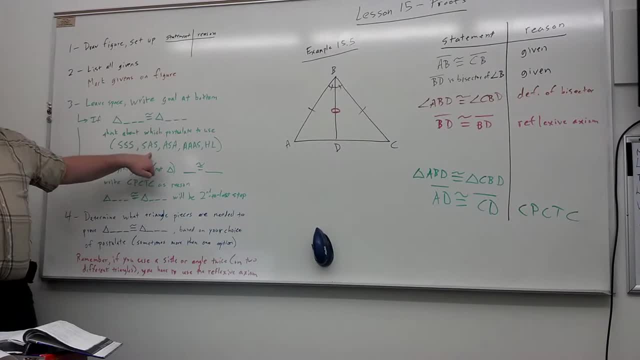 in order to use, in order to use the scheme, it has to be the angle between the two sides. It is, And it is So. there is our reason. So we've determined what we've determined what pieces are needed to prove our two triangles. 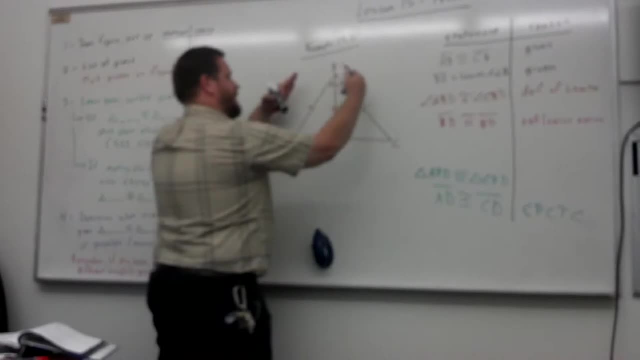 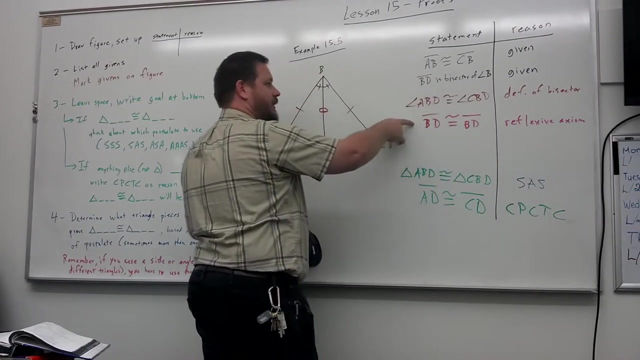 And we decided to use. we decided to use SAS And we have side, angle, side, And so the reason that these two triangles are congruent is SAS, which we can say now because we've, because we've made these two statements. 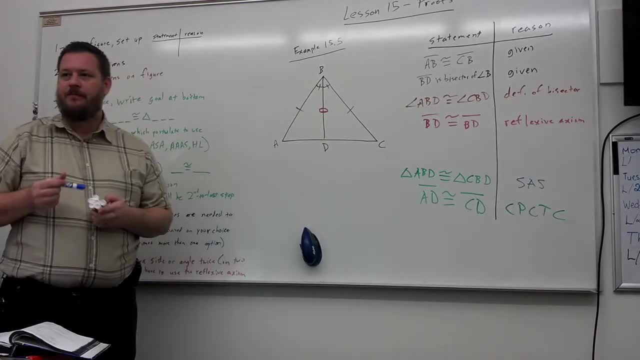 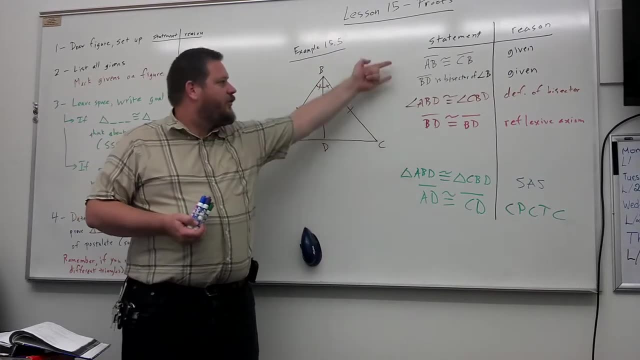 And We're done with this proof. So, even though it looks pretty big and scary, you know one, two, three, four, five, six and you have. you have six lines. two of them came. the problem just gave you. 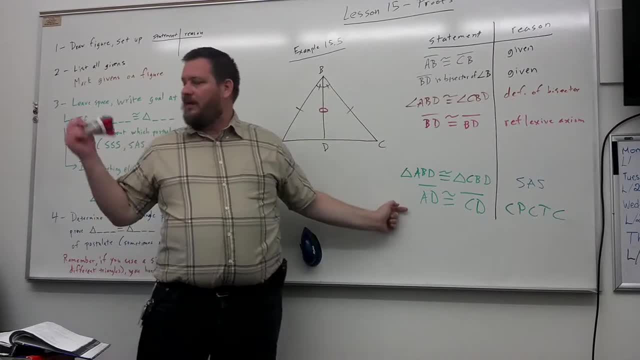 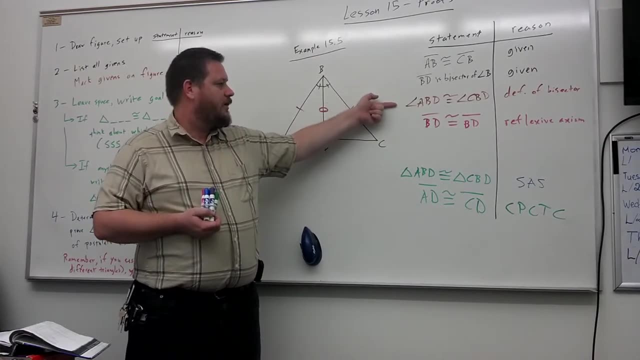 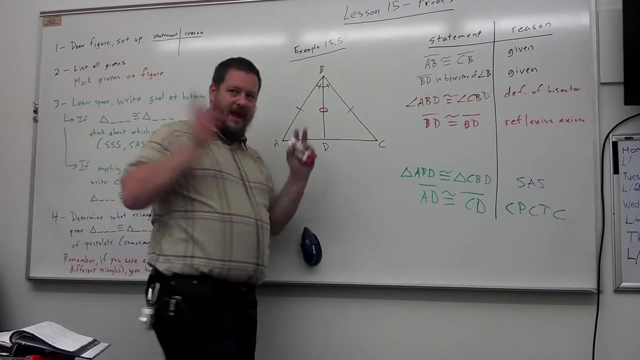 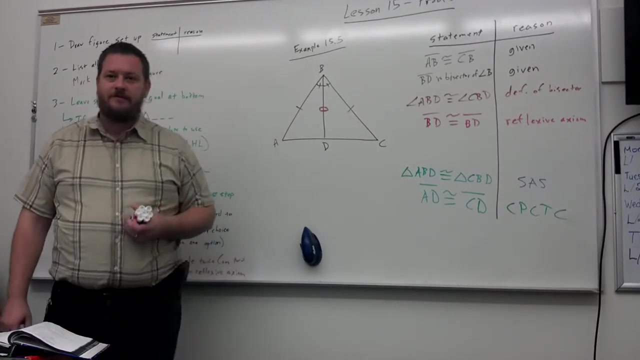 and this is what it asked for, And based on what I'm telling you, to tell you, And in case you're wondering, the answer to the question is this whole two-column chart, And so there is example 15.5.. Okay, 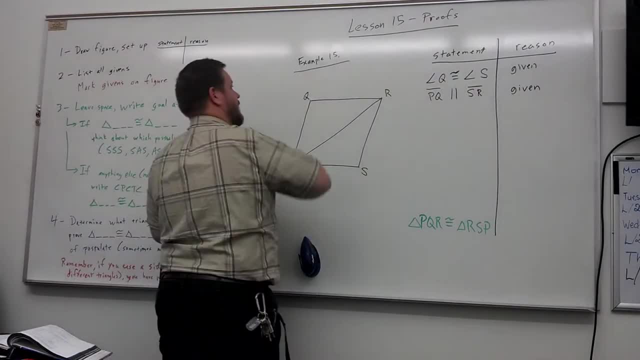 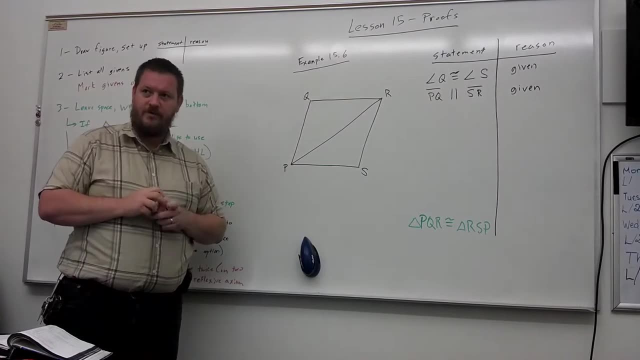 All right. So example: 15.6.. Oops, I forgot the label, It was 15.6.. Here's our shape And I've set up our the, the, my two-column proof. So I've, I've drawn, I've copied the figures in the book. 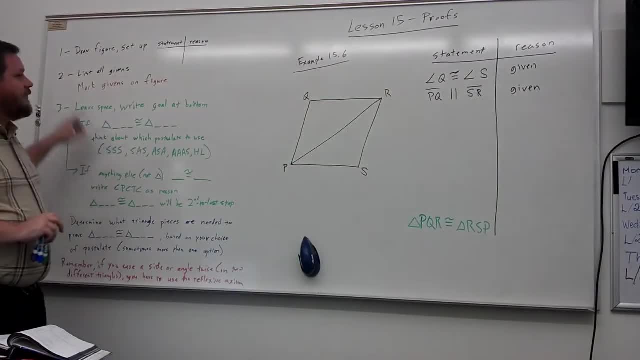 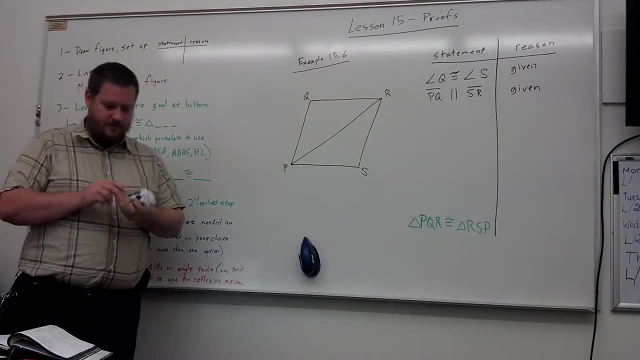 I've set up the two-column statement and reason. statements and reasons. I have listed the givens right here, So next next thing to do is I'm going to mark the givens on the figure. Since I'm color coding this, I'm going to use black or brown. 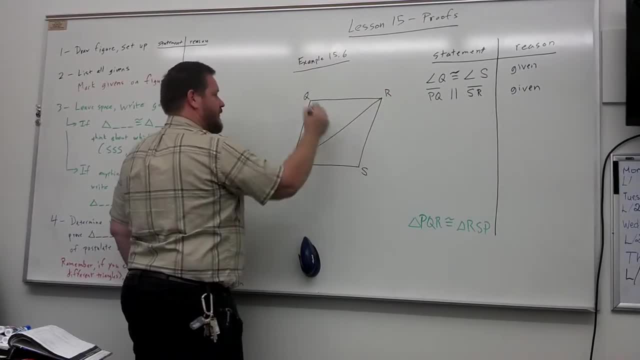 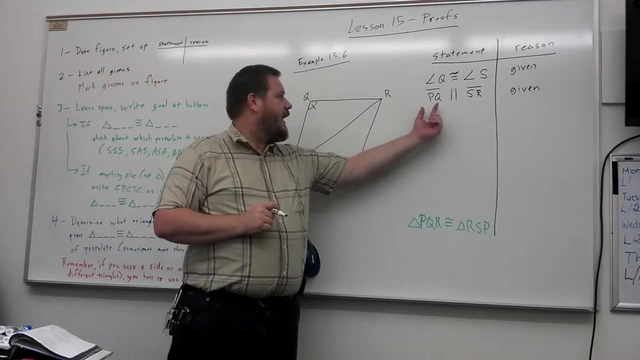 All right. So what are we told? Angle Q is congruent to angle S. So I know that this angle is congruent to this angle, because I was given that information, And I'm also told that line PQ is parallel to SR. Notice the order. by the way, 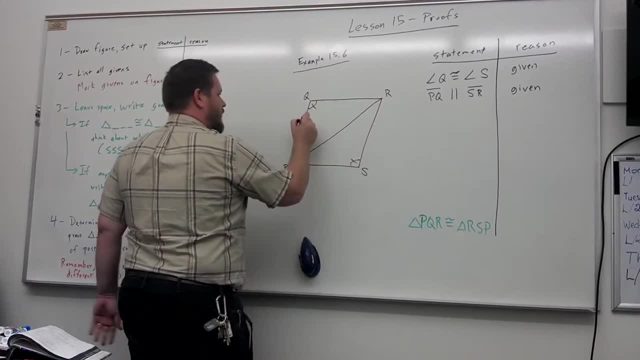 PQ is parallel to SR, So I know that these two lines are parallel And that's what I've been given. Wow, Pretty amazing stuff, huh. Here's a little tip: Any time you're told that there are two parallel, that two lines are parallel, sometimes it helps. 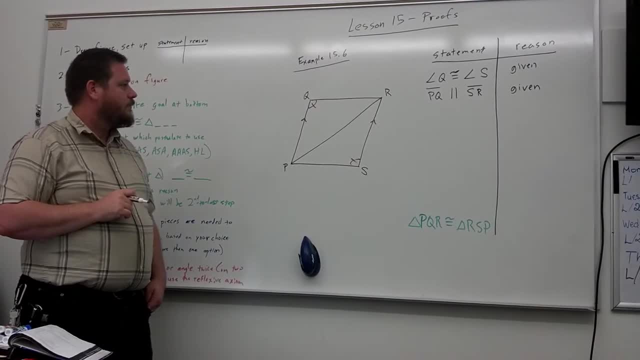 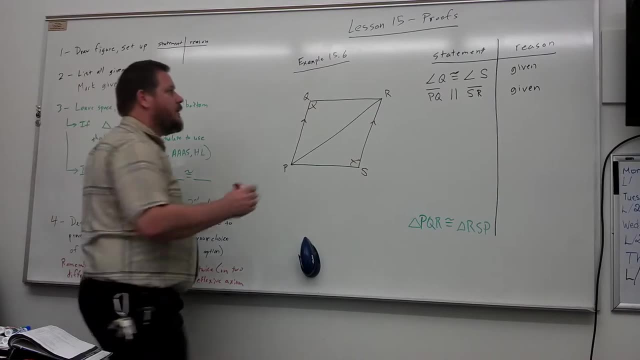 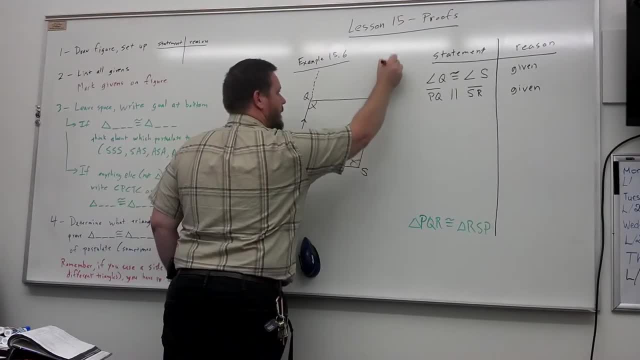 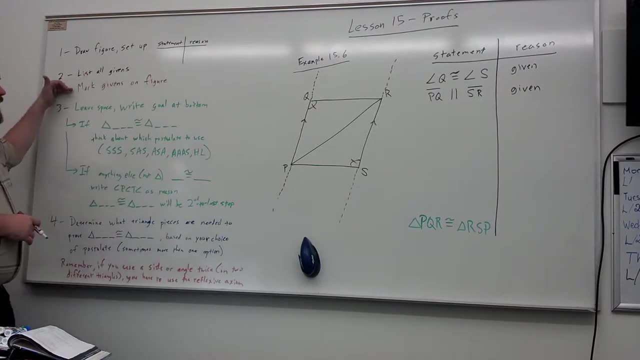 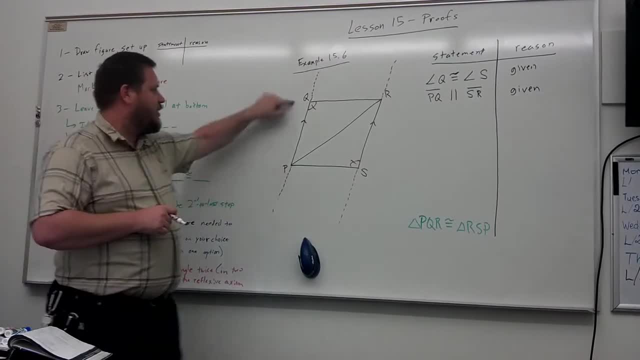 All right And so okay. So I've marked my givens on there And now I know what it is. So I left a space And my goal at the bottom of this one is to prove that these, that triangle, PQR. 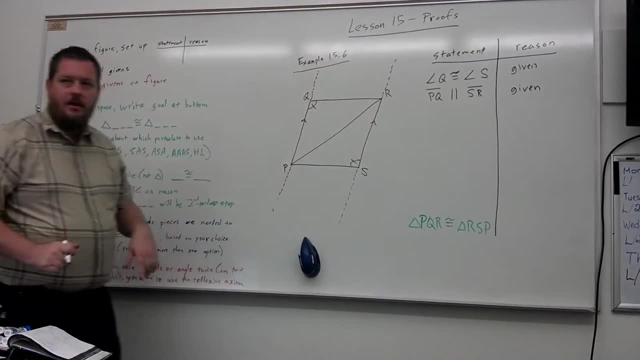 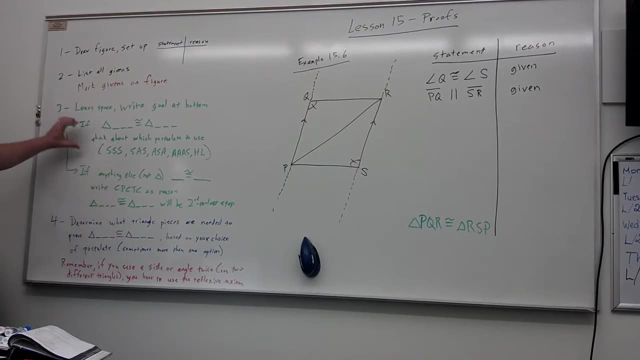 So that this triangle right here is congruent to RSP. this one here. And, like I said, there are two types of proofs that you will encounter in this book. We did the other one on the example 15.5.. This one falls into this category. 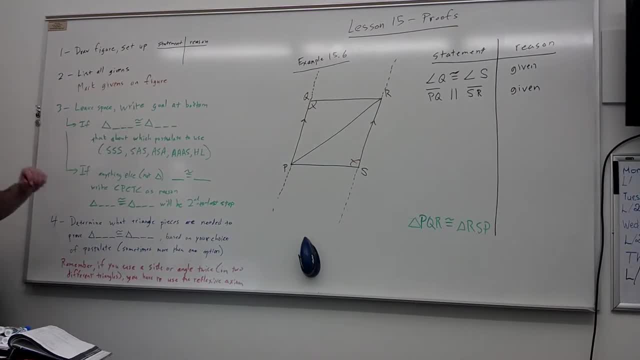 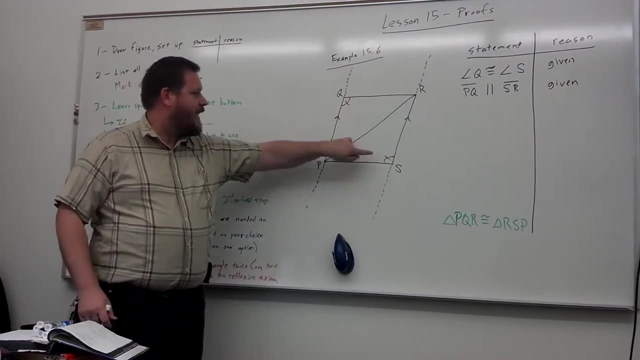 We are trying to prove that two triangles are congruent to RSP. triangles are congruent. therefore, we need to figure out which postulate we're going to be using. Now we are all. we are already told that these two angles are congruent. 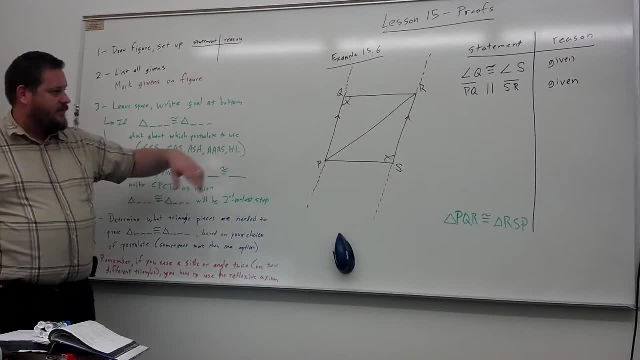 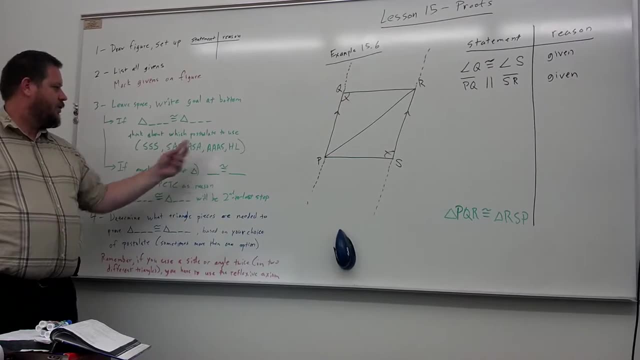 so we're probably not going to use SSS And, from the look of things, these are not right triangles, so we're not going to be using HL. That leaves these three And, like I said, this one is you. usually you can do one of these two, SAS or ASA, And so let's, let's aim for one of these. 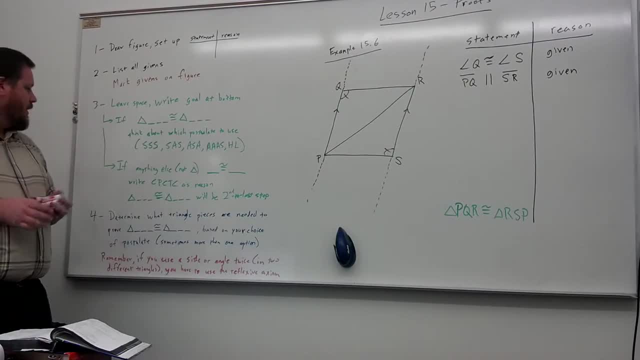 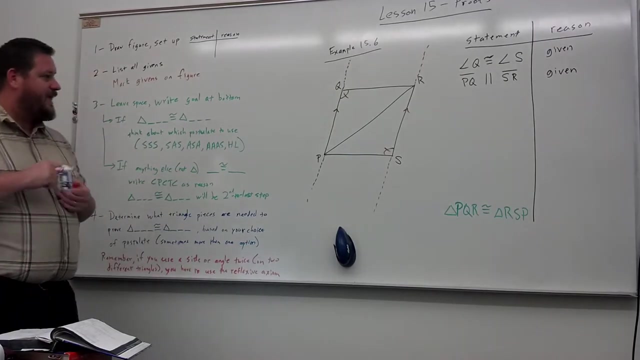 three and see what we- what we can find out from that- Just as a quick idea here- are we going to use. do you think we're going to use anything twice in both triangles, Or do something twice once in each triangle? What Line PR is in both triangles? So line PR is congruent to line PR. 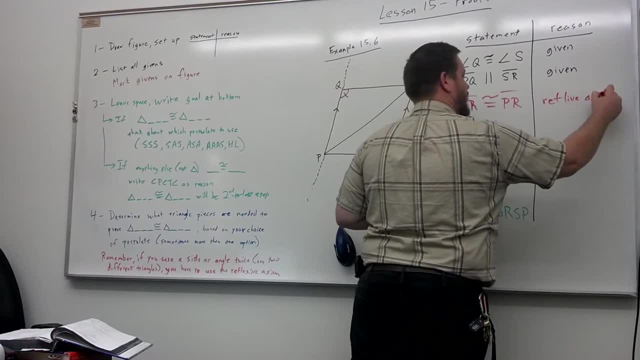 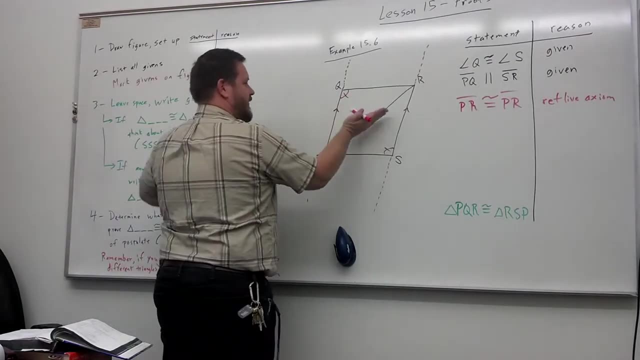 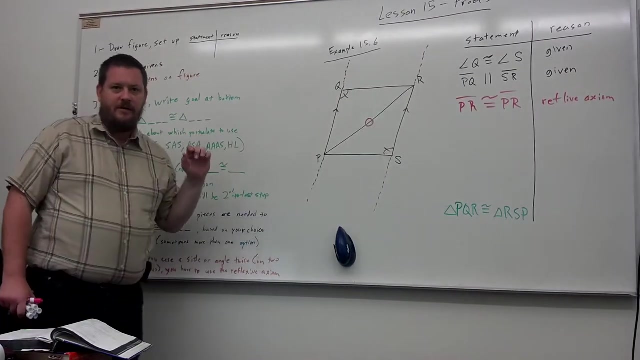 and that's the reflexive axiom. I'm going to go through a little circle here. So we've got an angle and we've got a side. Now notice that the angle is not next, the side is not next to the angle. So that means we might end up having to do AAAS. 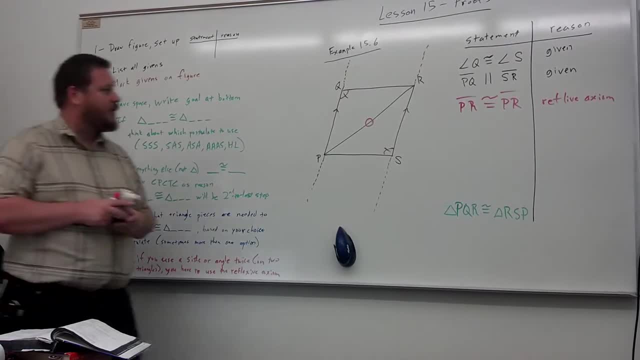 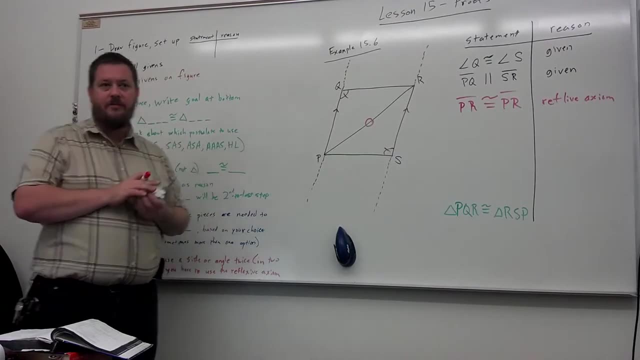 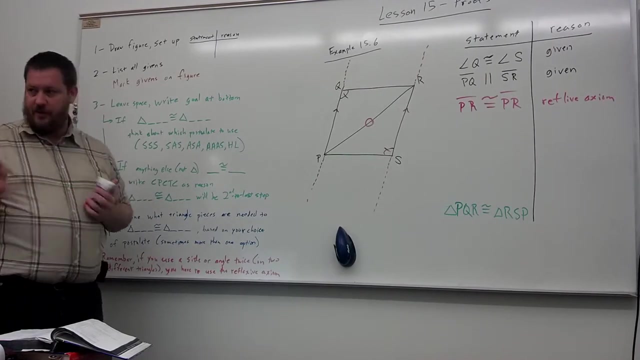 possibly, So let's keep our options open here. Now, what do we know here? What else can we, can we look for? We need to find something about either a pair of angles or a pair of sides. No, You know vertical angles. There are some problems that we do Vertical angles. 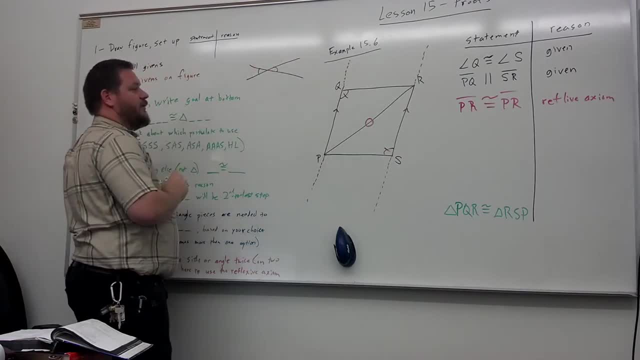 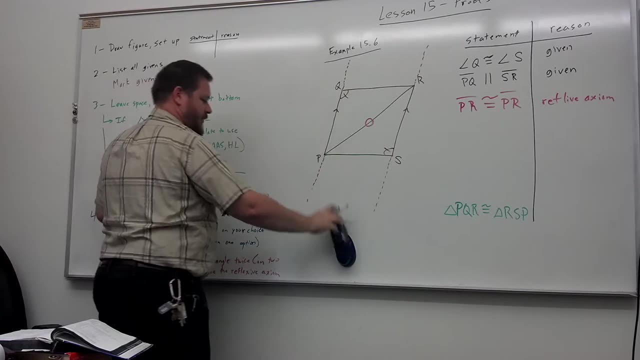 are when two lines cross, and you're talking about those angles right there. Ah, I than we-and we don't- clearer ahead. We could make vertical angles, but I don't think we need two of those crossed. You notice anything? Is there anything else we can do? 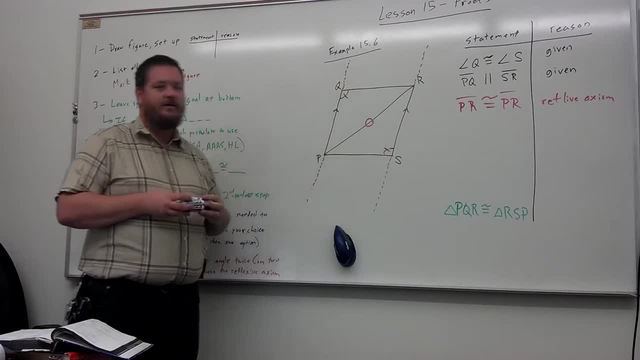 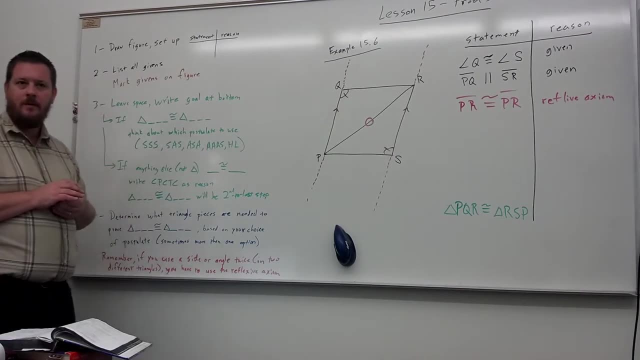 Remember I said: anytime you have parallel sides, extend those sides out, three into one sides out, and see if that helps to notice anything. Extending those, Oh, maybe P R or P S, That's given P S and Q R are parallel. 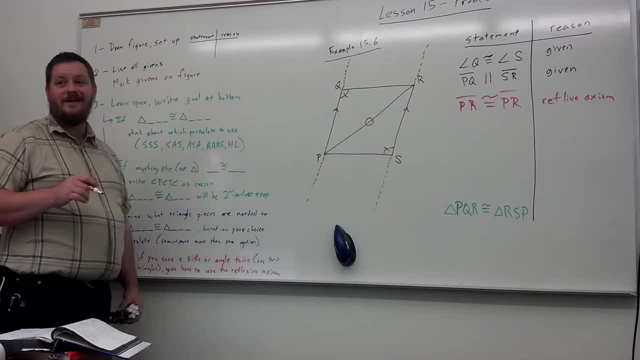 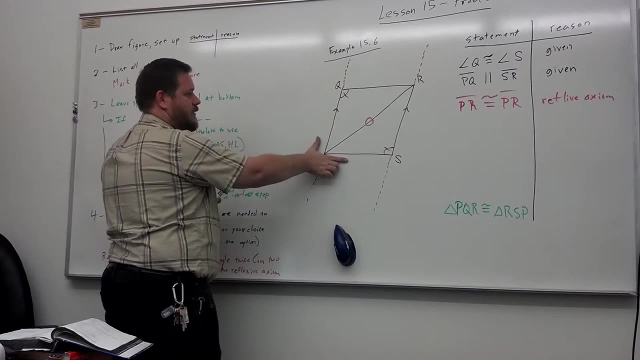 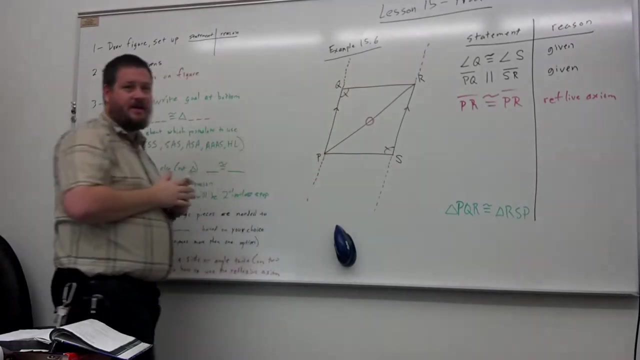 They're the same length. We don't know that yet. What did you say? Angle P or angle R? Angle P- Angle R? You could only say that if you knew that these two were parallel, then you could say that. 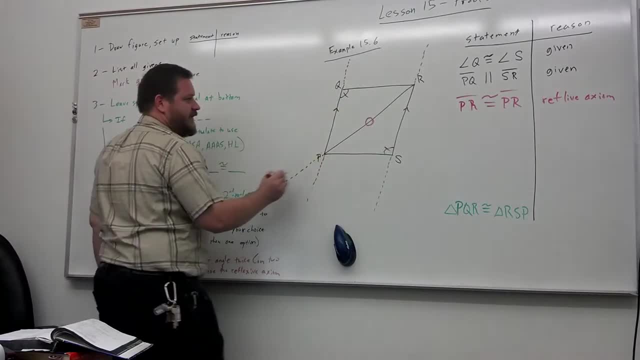 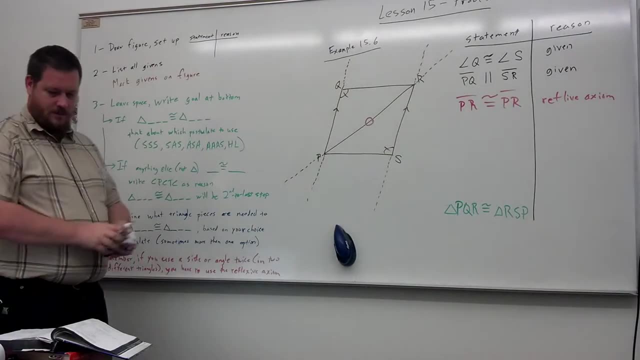 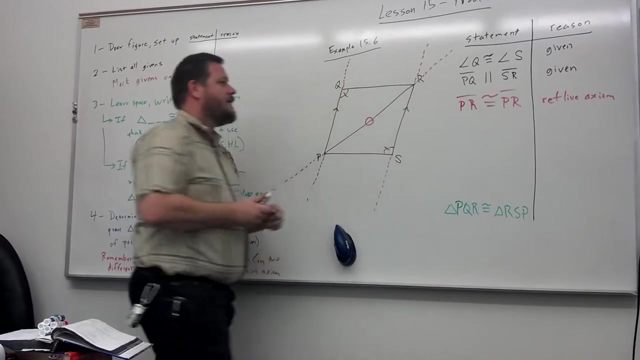 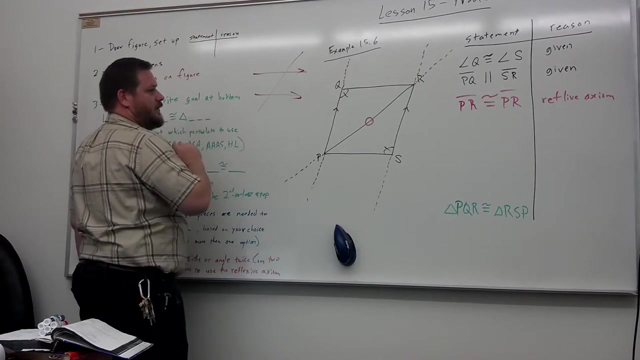 Let's take this P R line and extend it also Angle Q P R, So Q P R S R P, Because anytime you have parallel lines that are cut by a transversal, the These two angles like this: 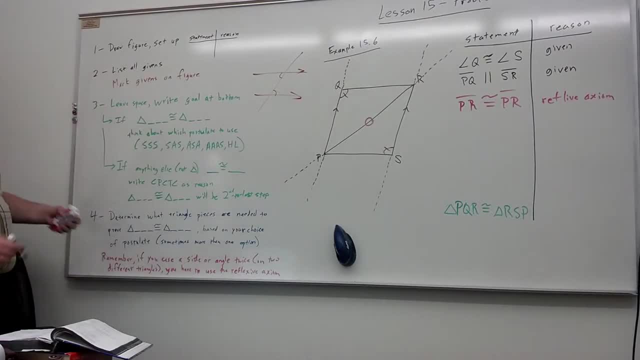 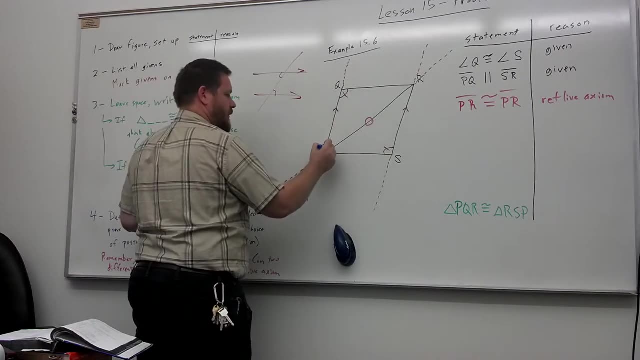 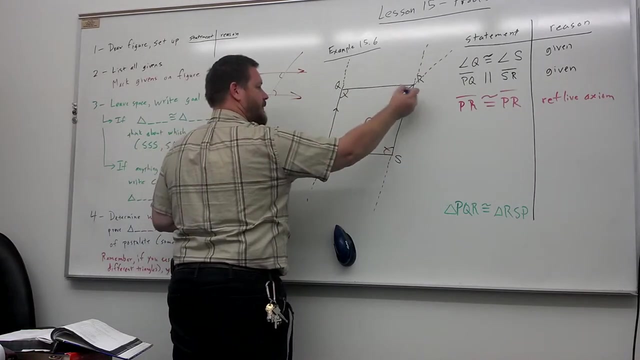 Alright, We're working in blue now. So you want to say that? What did you say? Q P R. So this angle right here. That's what you said, right. And then S R P, That one there. 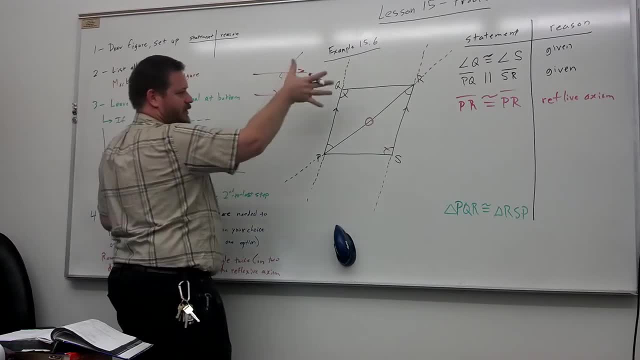 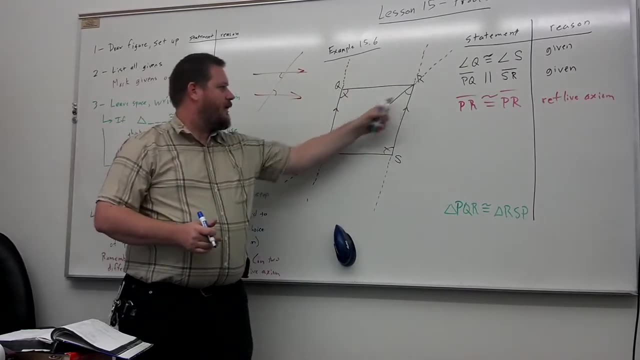 Everybody see that. This idea, You've kind of got to turn it sideways a little, Oh, okay, yeah, If these two lines are parallel and this one cuts through them, these two angles are going to be congruent. I've already used one tick for angle, so I'm going to do two ticks here. 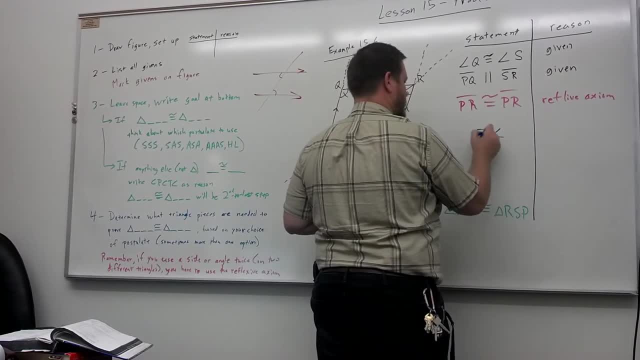 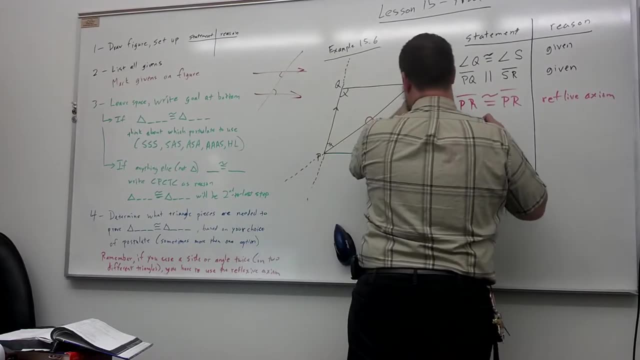 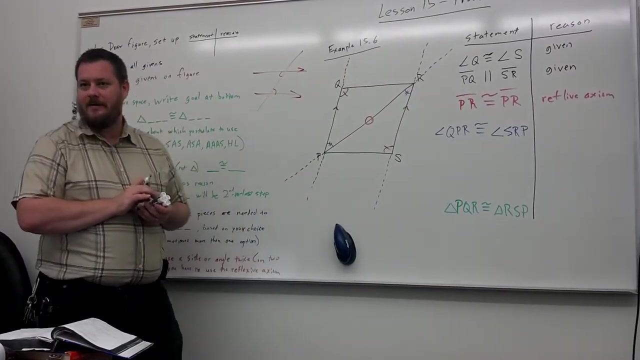 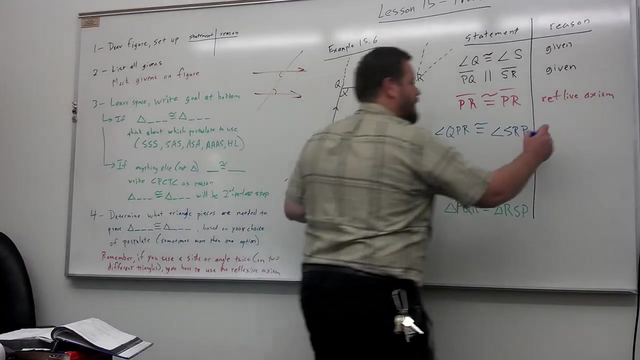 So we've got. So angle Q, P, R And then S R, P. Those two angles are congruent. Why? Because of this right, What we call these are, When you have like this, these two angles are called alternate. 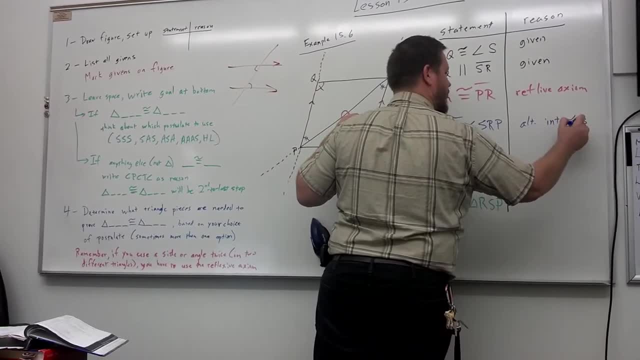 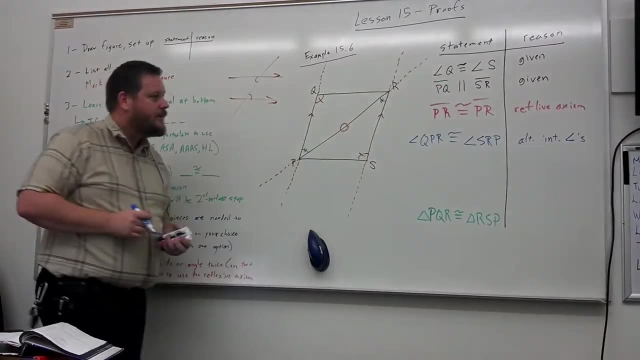 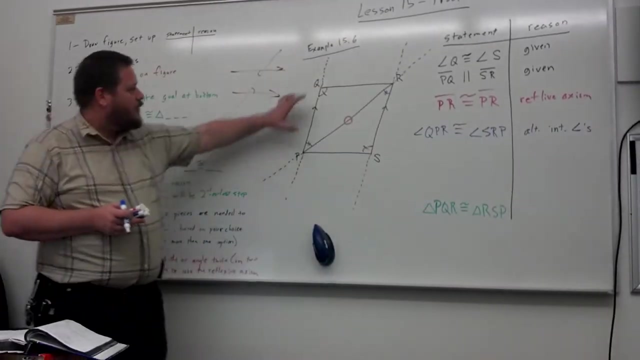 interior angles, And you can abbreviate as much as you need to over here. Just make sure that it's clear what you mean: Interior angles. Now do we have enough to say that the triangle is congruent? No, We've got two angles and a side. 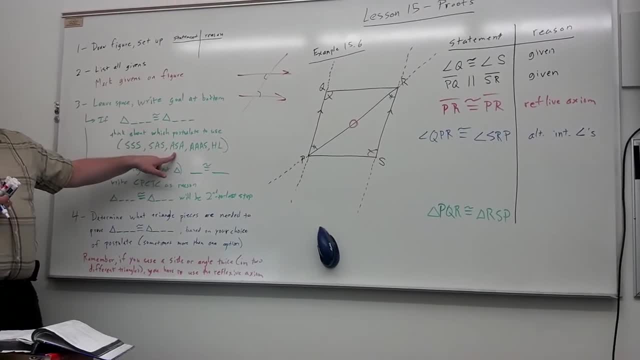 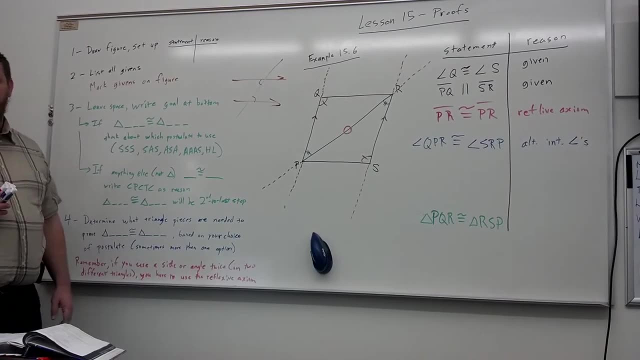 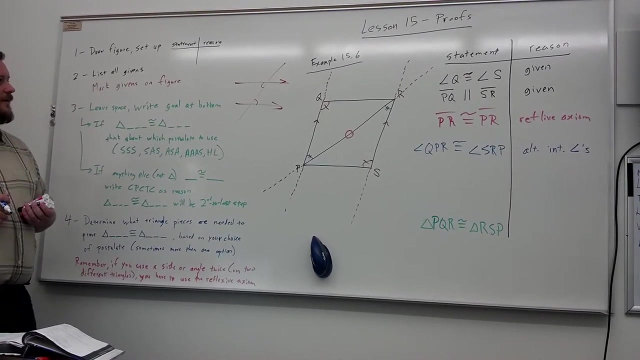 No, Can we use ASA? No, No, Why not? We need another side. Yes, the side is not between the two angles, So we need something else. Q R P is anterior to the side, That's right. 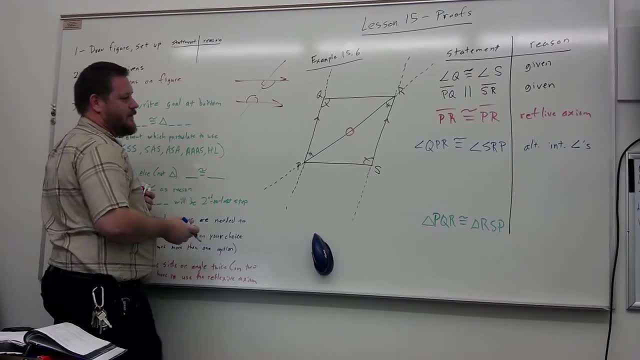 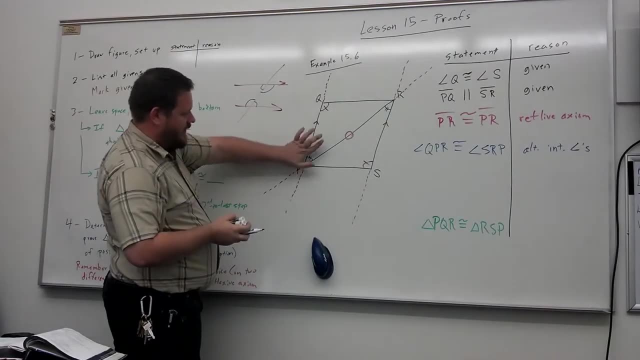 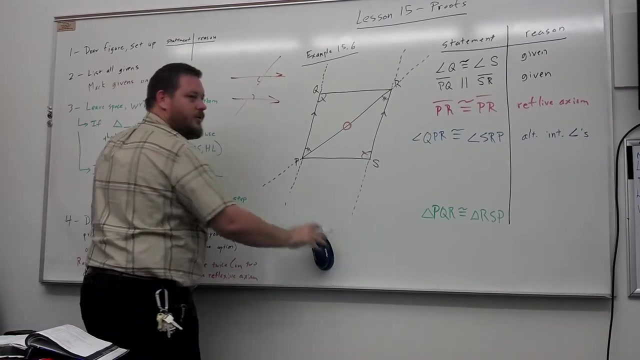 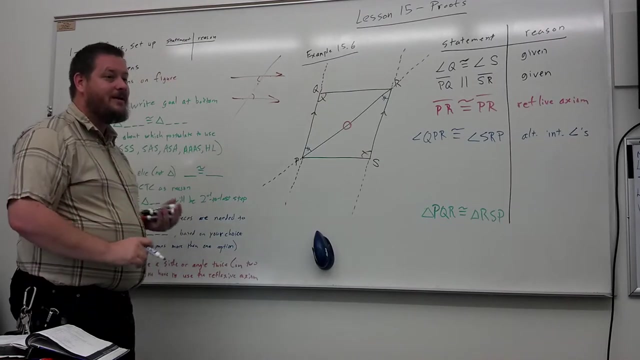 For the exact same reason, we can do the other pair. Oh wait, Hold on. Actually, No, we can't, Because that's this one, not this one. We can't do that. What Yes? Why? Because what Yes. 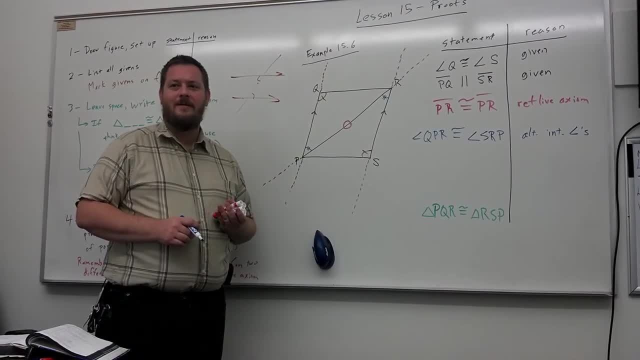 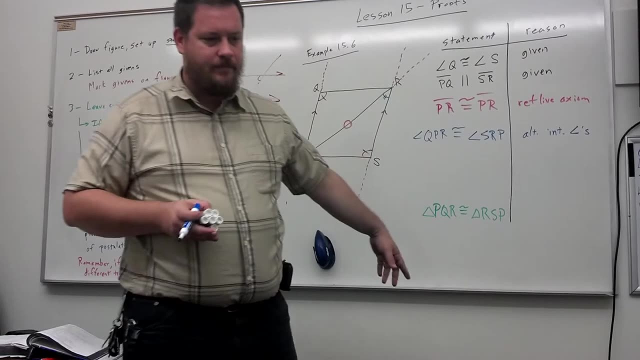 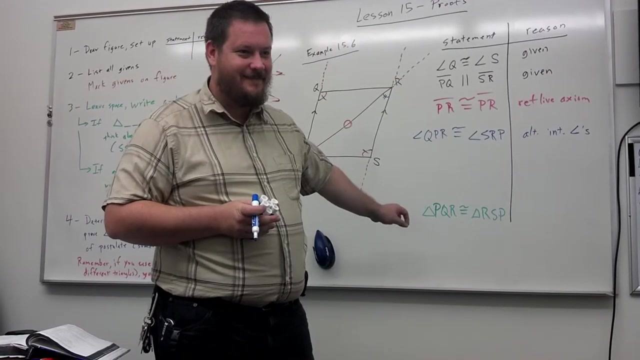 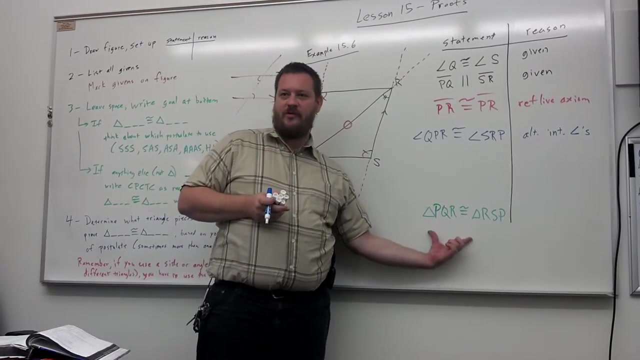 Why are you talking back there? Because I dropped something. Okay. What shapes are we talking about here? Now is not the time to be texting, All right. What shapes are we talking about? Triangles, Triangles. How many angles in a triangle? 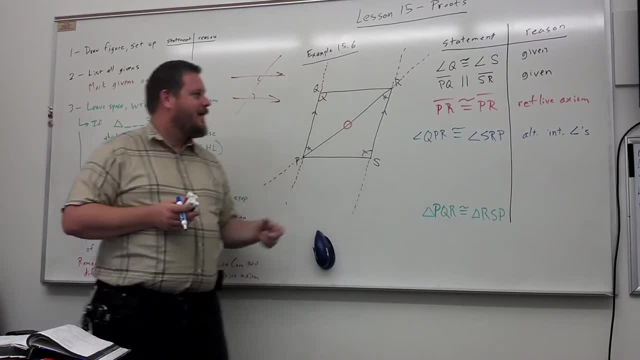 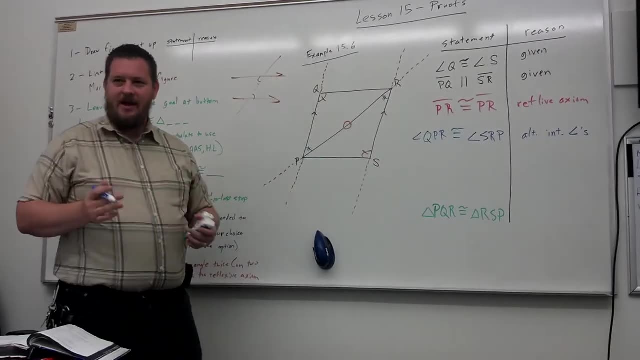 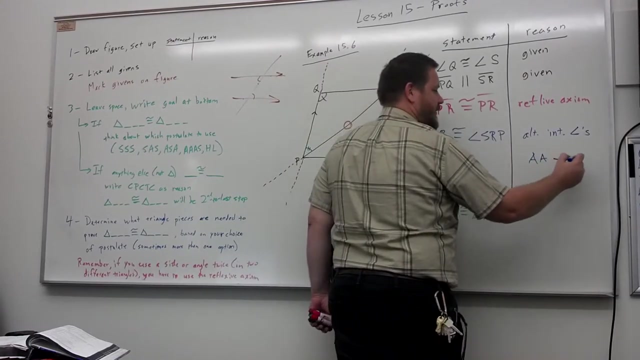 Five, Three- How many do we have so far? We know this pair and this pair And if there's only three angles in a triangle, any time, you know that two angles are the same. therefore, all three angles must be the same. 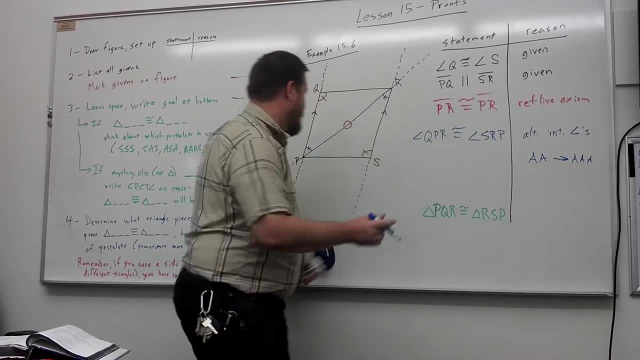 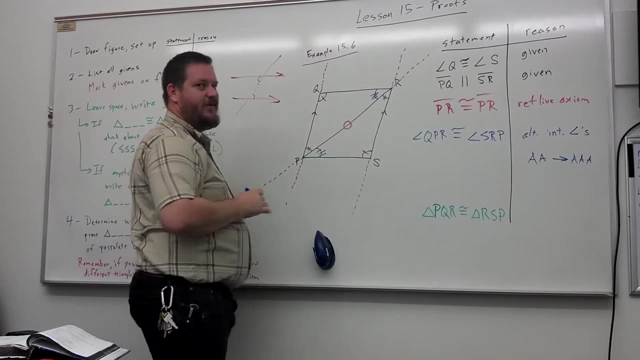 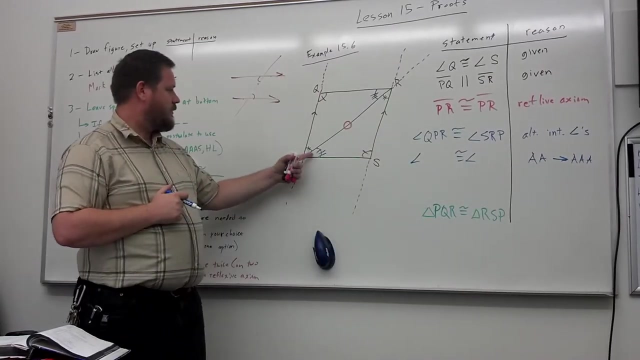 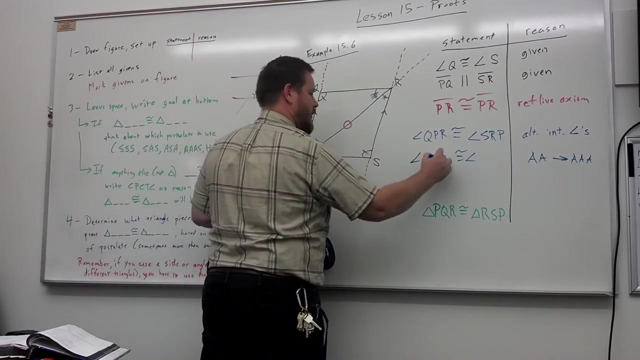 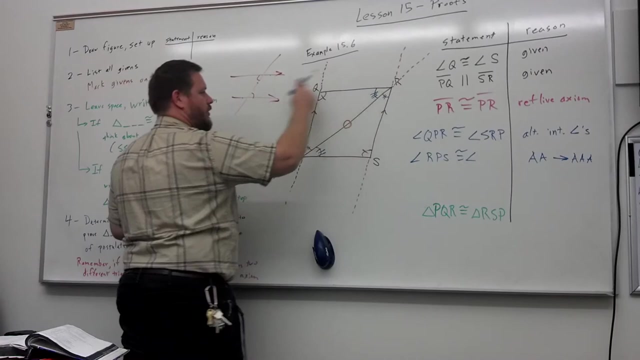 I would read this as AA means AAA. So therefore the third angle must be congruent, because the other two aren't. So this is angle. What should we call this angle RPS? It's got to go the same order for this one then. 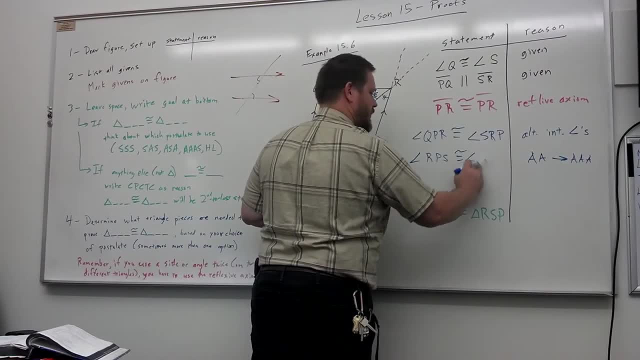 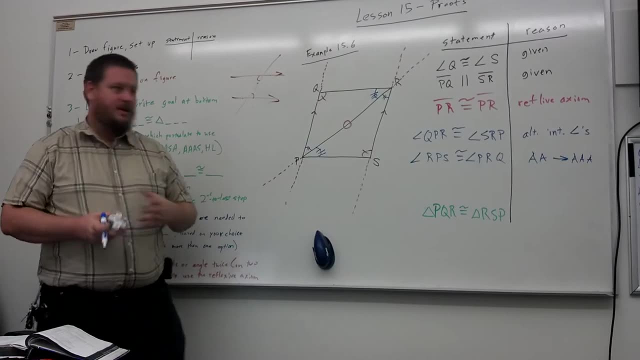 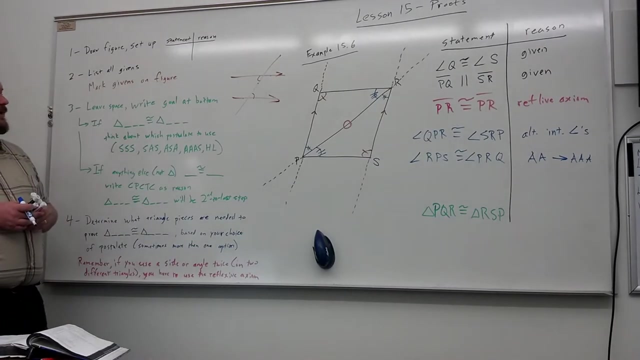 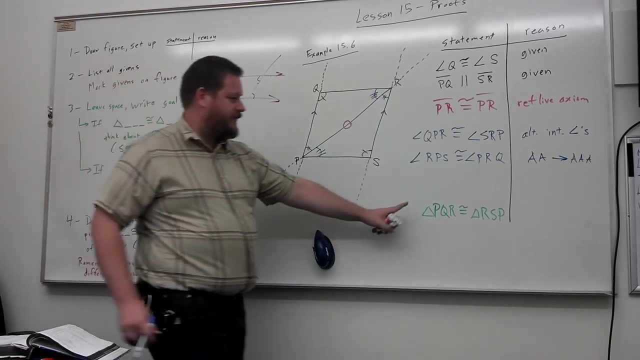 Now PRQ, PRQ. So these two angles are congruent. because when two angles are congruent, then the third angle must be congruent also. Now do we have enough proof? Yes, Now we know all three angles plus a side. So now we have enough to prove that the two triangles are congruent. because of what reason? 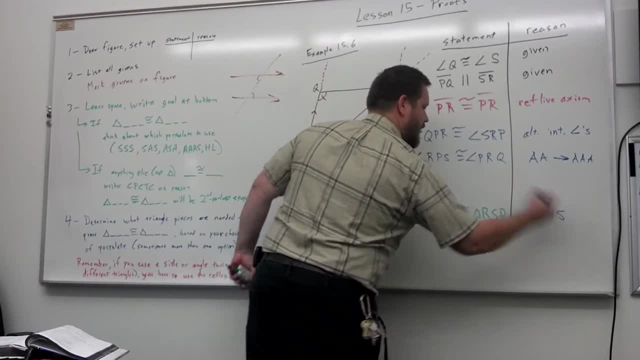 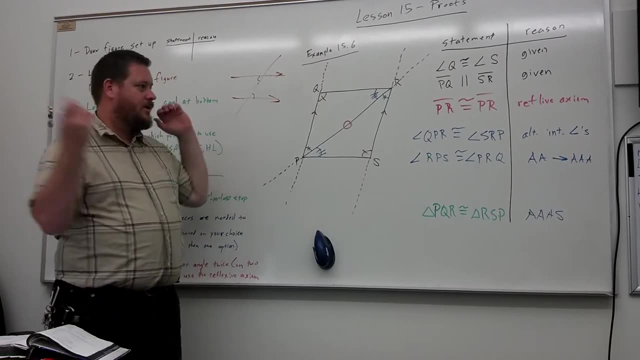 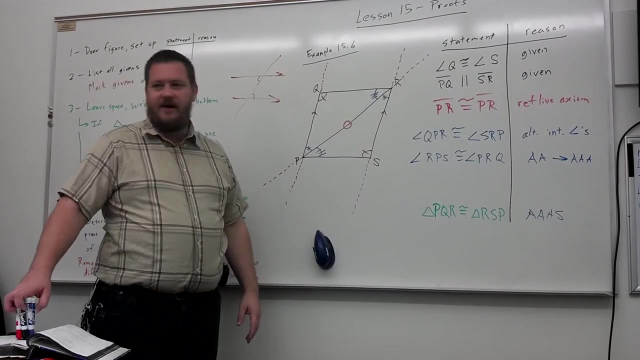 AA, RPS. And there you have it. It takes a little bit of getting used to getting the hang of it. Personally, I find these problems irritating just because I don't like to do that much writing. But once you get the hang of it after a few of them. 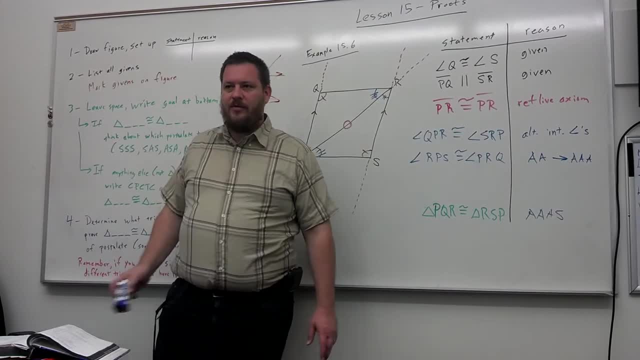 they're not all that difficult if you remember the basic idea of what you need to do.